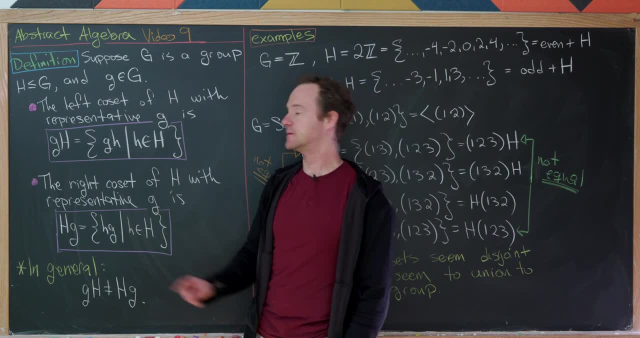 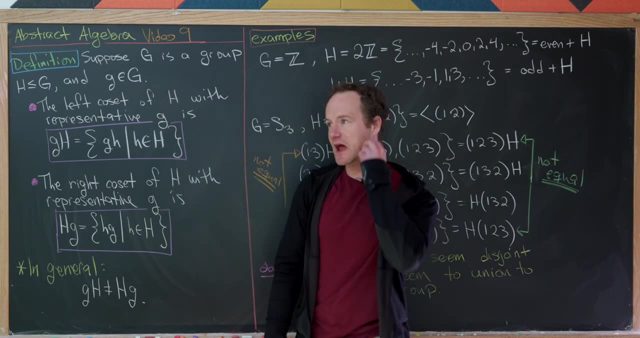 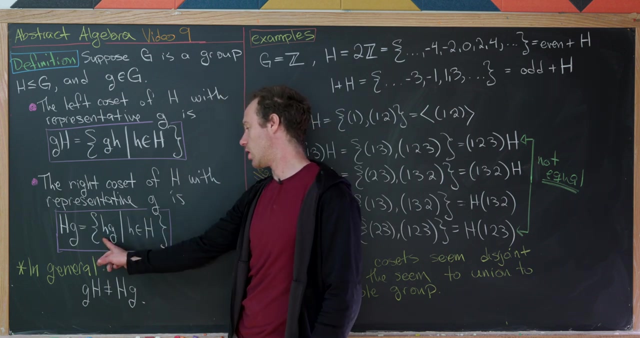 And that's what I have here encoded in this set builder notation. This is G times H, as H runs through everything from H. And then likewise, we could define something called the right coset, which is all right multiples of elements of H by G. And like I said, that will be H G, where that's the set containing all little h times little g as H runs through all H. 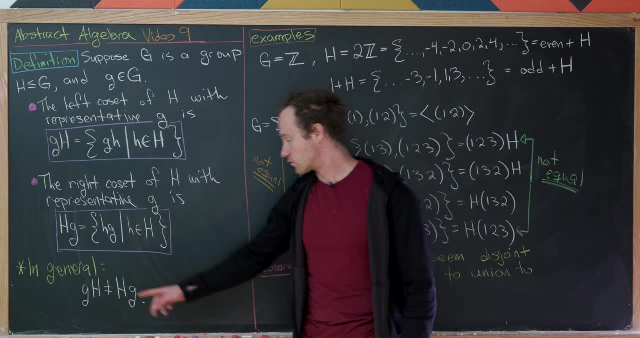 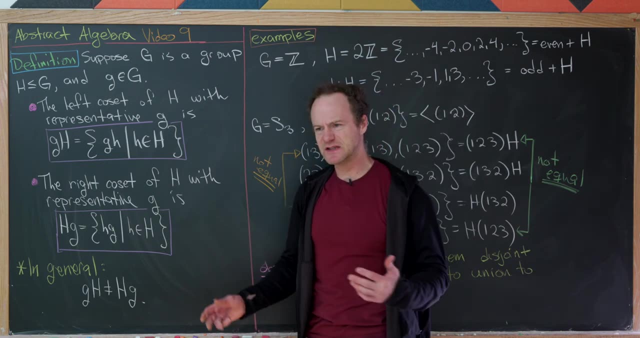 And I'd like to point out here in general that right cosets are not generally equal to the corresponding left coset. And that's because generally we don't have commutativity in groups. But we will see cases when these are equal even outside of abelian groups. 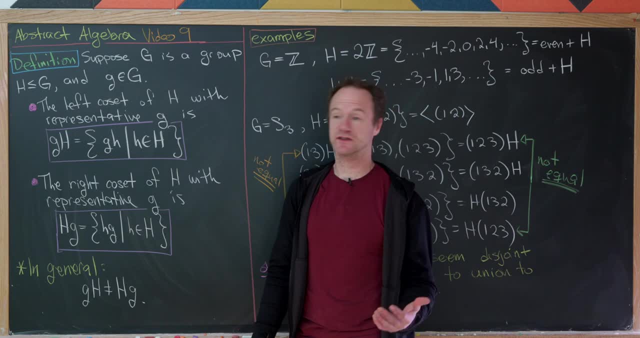 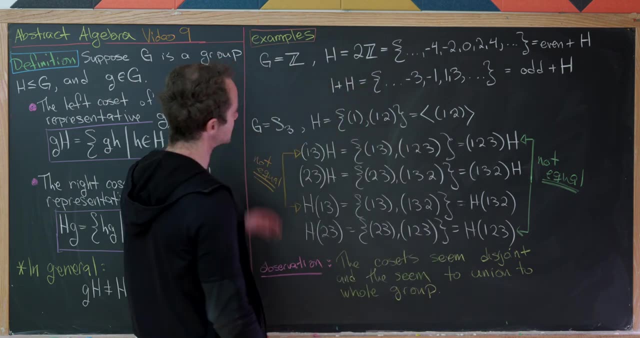 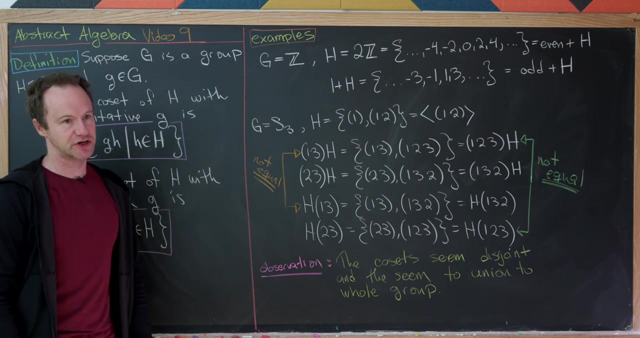 And that'll actually be a really special case of a subgroup. Okay, so anyway, we've got G H is in general not equal to H G. Okay, so now let's look at some examples. Maybe this first example, which is a cyclic group is a subgroup. So let's say that G is the additive group of integers, and then H is the cyclic group generated by the number two. So let's recall that we wrote that as 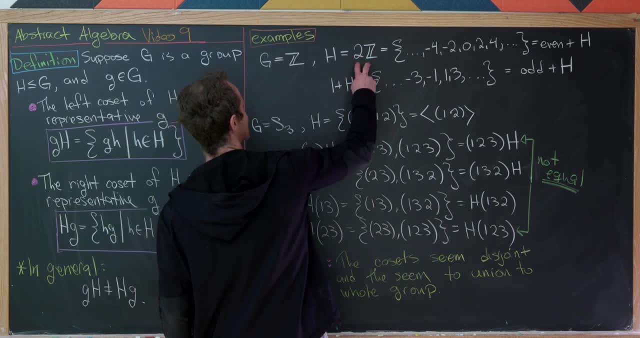 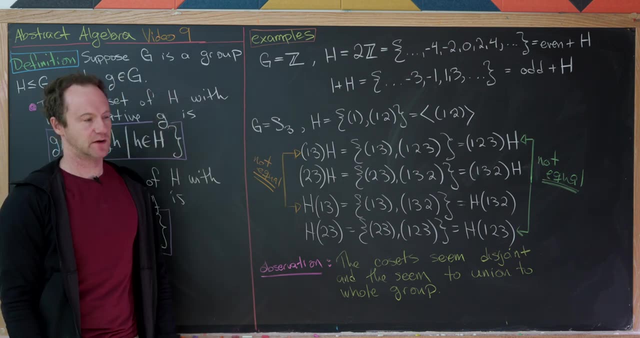 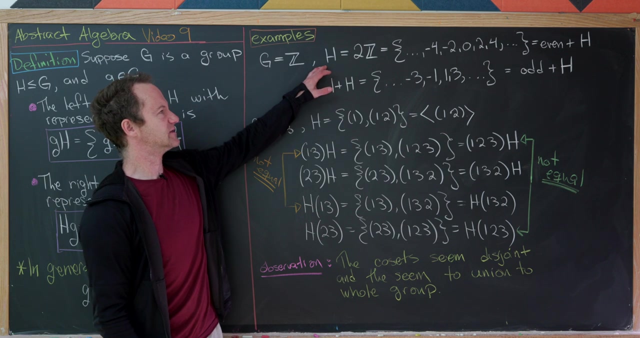 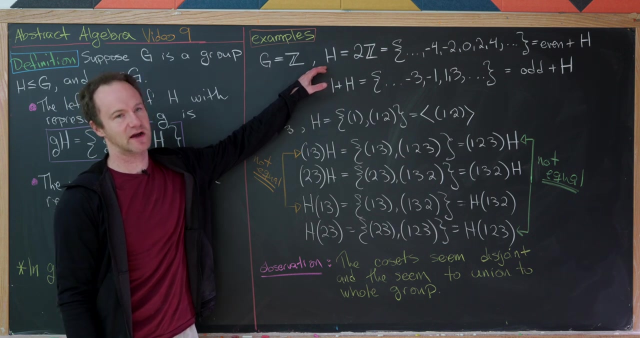 two times Z, and that was simply all even numbers. And we talked before why that forms a subgroup, but since it's a cyclic subgroup, it's obviously a subgroup. But I'd like to point out that in the subgroup. But I'd like to notice that this is maybe its own coset with multiplication by the identity. I shouldn't say multiplication here, operation by the identity. Our operation is addition. But since if we add any even 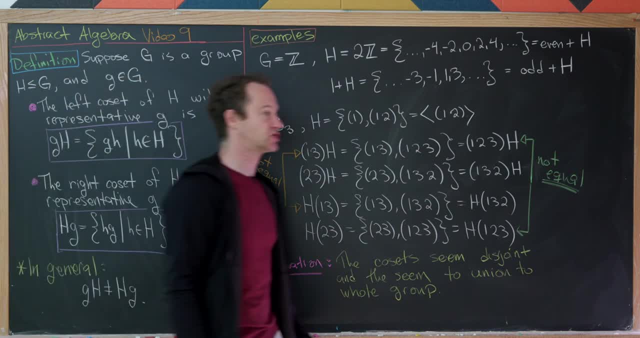 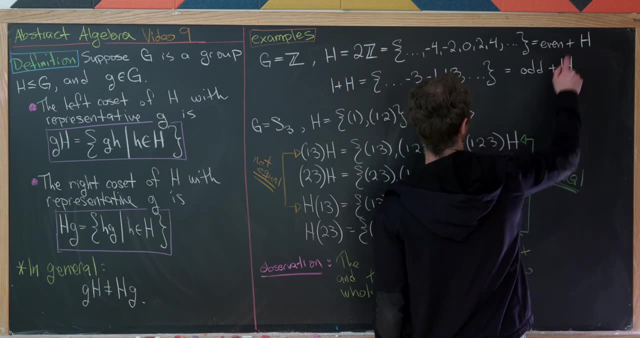 number to an element of H, we land back in H, we actually have, this is the coset connected to any even number. And let's notice here that I'm using the plus symbol because we have plus as our operation. So for abstract groups, we'll 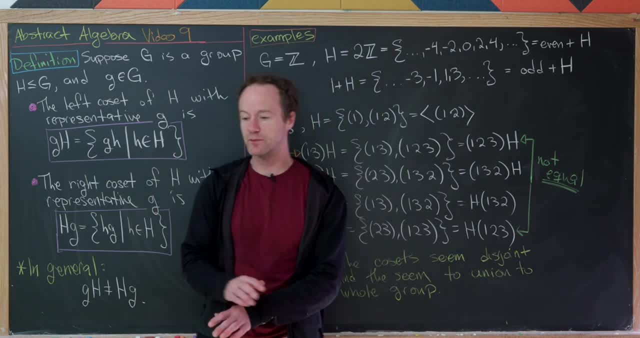 just put them next to each other and read it as multiplication. But if we know the operation, we'll use that operation. And in general, that most of the time 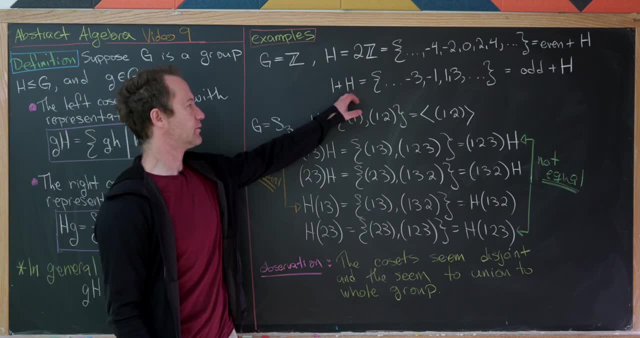 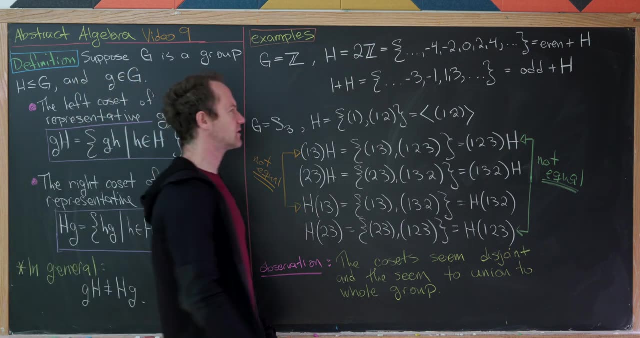 will be when we have addition. Let's also notice that 1 plus H will be the set containing everything in H plus 1. But that'll give us negative 3, negative 1, 1, 3, so on and so forth. 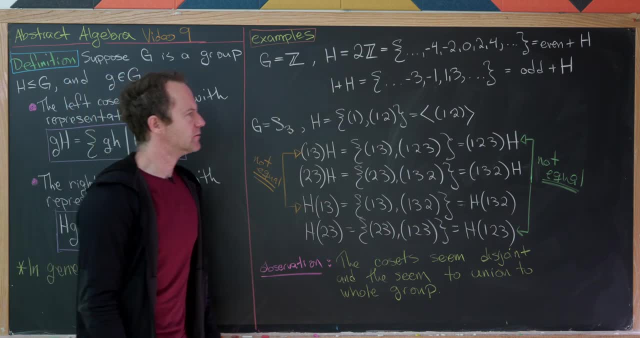 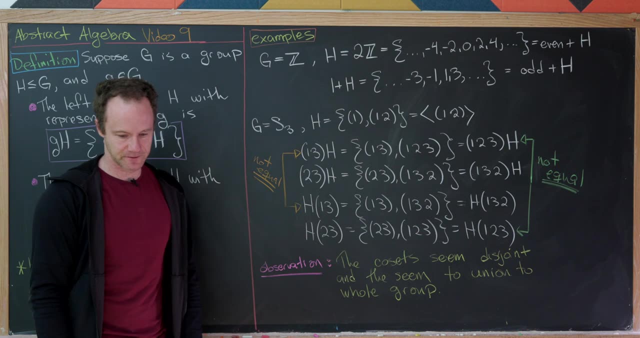 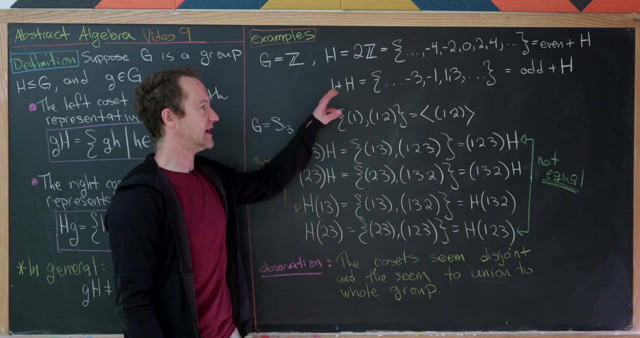 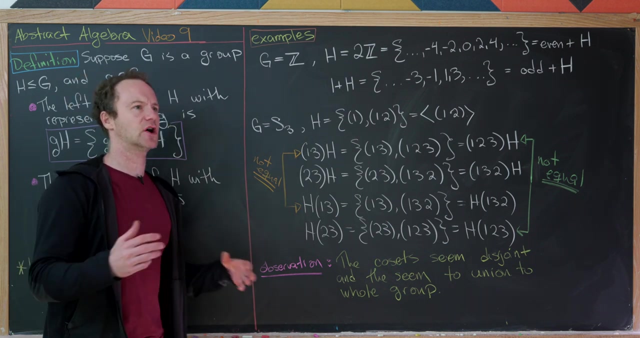 In other words, all odd numbers. But that's the same coset as the coset with any odd number plus H, just by the structure of H. Okay, so we have H is the subgroup of all even numbers, and its only coset is the odd numbers. It's no longer a subgroup though. So this sort of look at cosets is really a generalization of breaking groups into even and odd parts. 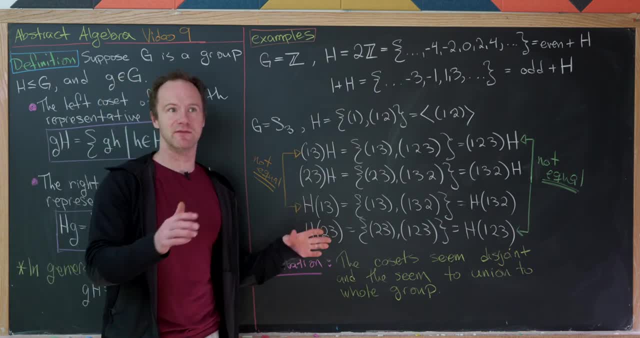 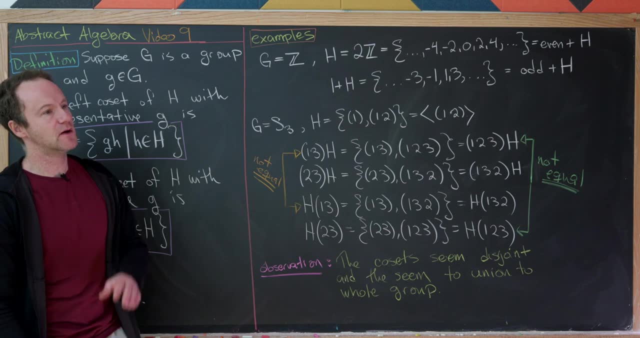 But we may have more than just two parts. It may be more than just even and odd. And in the integers, you can think of it kind of like congruence mod N, but we want to push it farther than the integers to general groups. 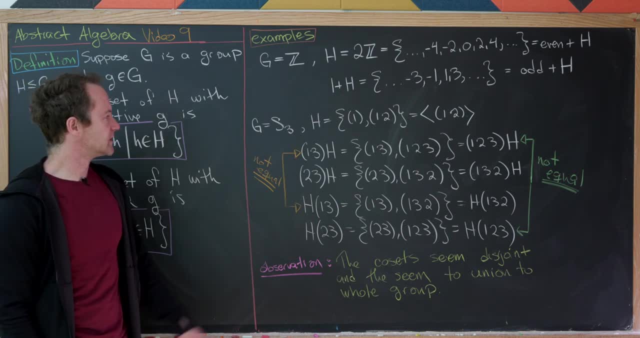 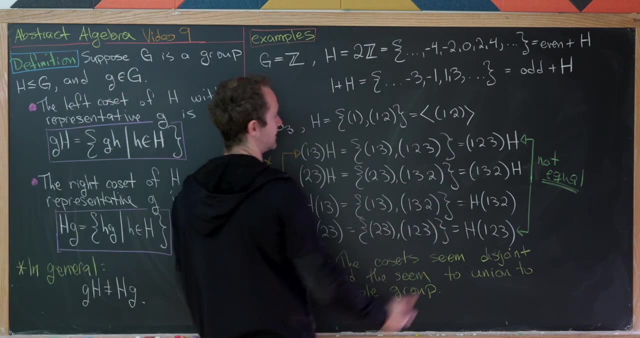 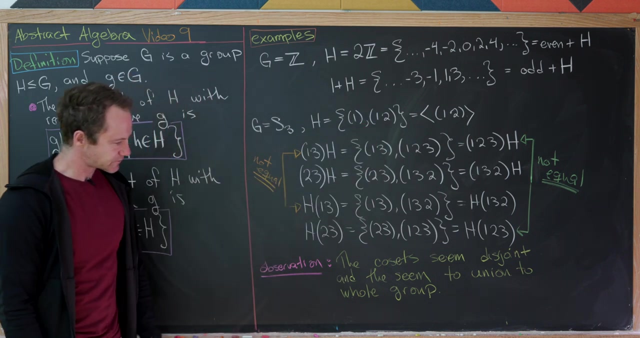 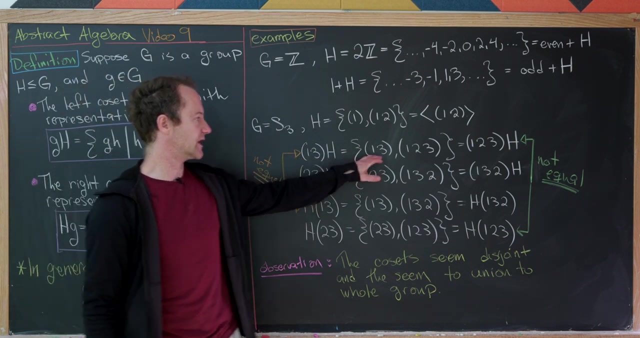 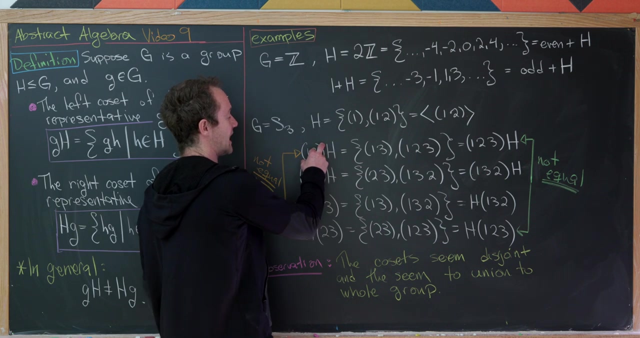 Okay, so let's look at another illustrative example. So let's take G to be equal to S3, and then we'll take H to be the cyclic subgroup generated by the two-cycle 1, 2. So that will contain the following two elements. The identity and 1, 2. Now if we were to do our calculations and calculate the left coset of 1, 3, H, we would get 1, 3, 1, 2, 3. And I'll let you calculate that out, but that's what you get if you left multiply 1, 3, and 1, 2. You get 1, 2, 3. 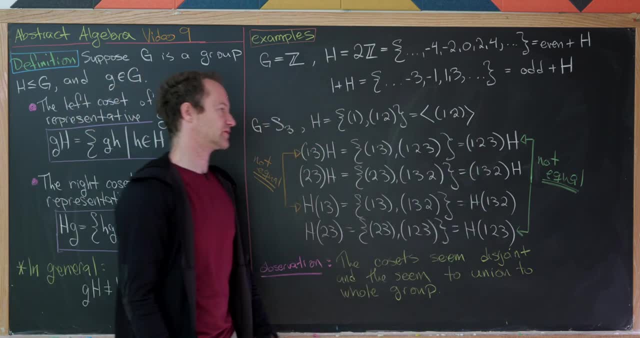 But that's the same thing as the left coset with representative 1, 2, 3. So 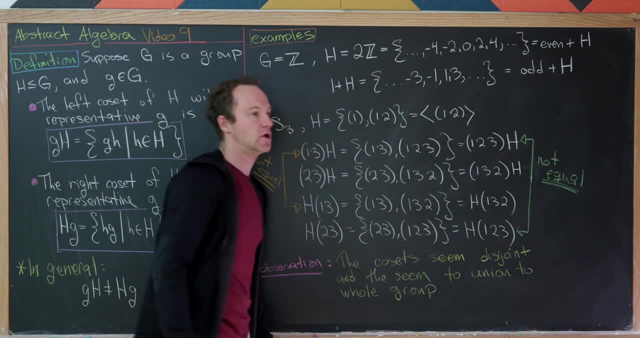 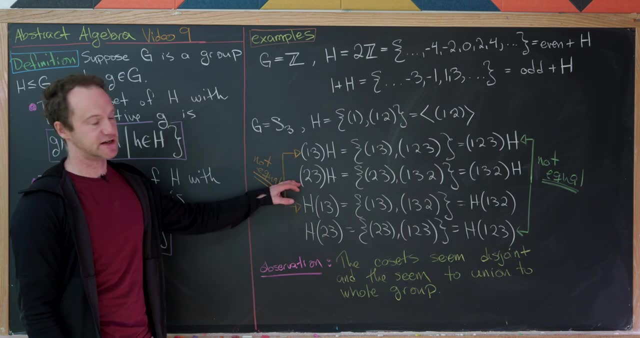 let's notice that two cosets can be equal with different representatives. That's why we've used the word representative here. Then the left coset associated to 2, 3 is the following set. So 2, 3, we get 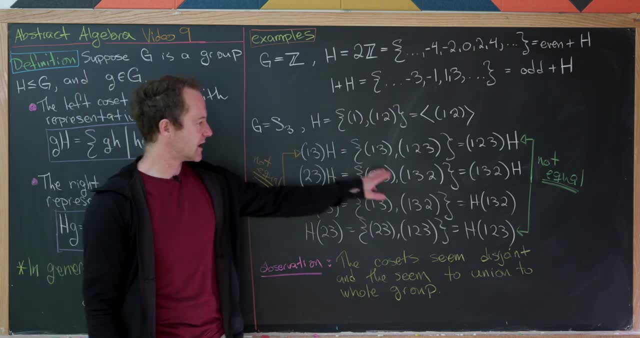 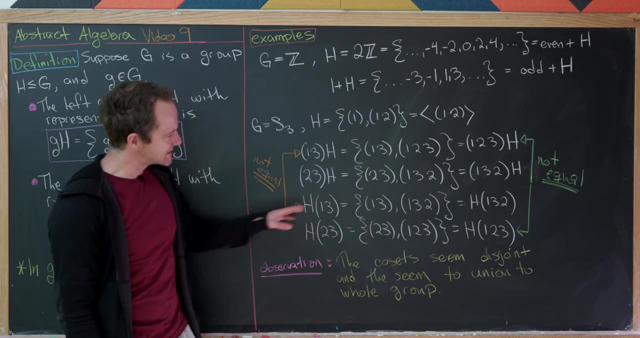 that from multiplying 2, 3 into the identity. And 1, 3, 2, we get that from multiplying 2, 3 into 1, 2. That's the same thing as the left coset of 1, 3, 2 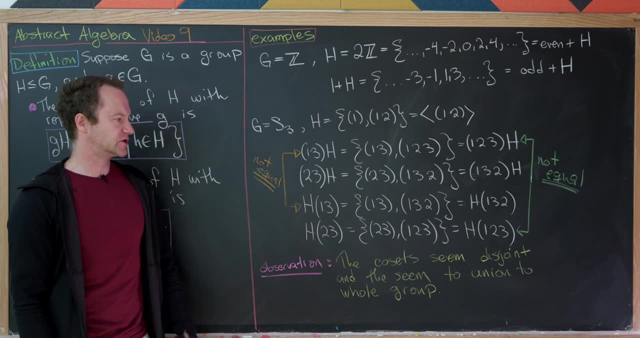 as well. But we have right cosets as well, which can be calculated similarly. Maybe I'll let you think about how these could be calculated. Maybe work the details out on your own. The most important thing to notice is that this 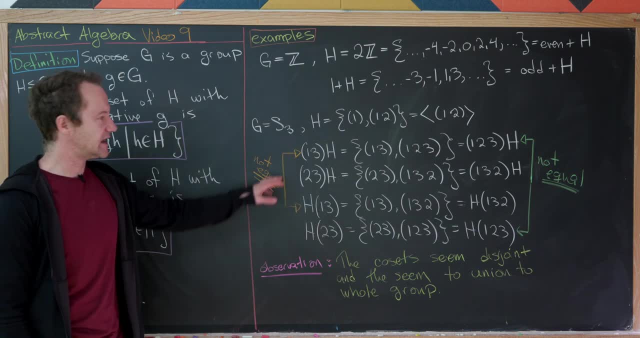 right coset attached to 1, 3 is not equal to the left coset connected to 1, 3. 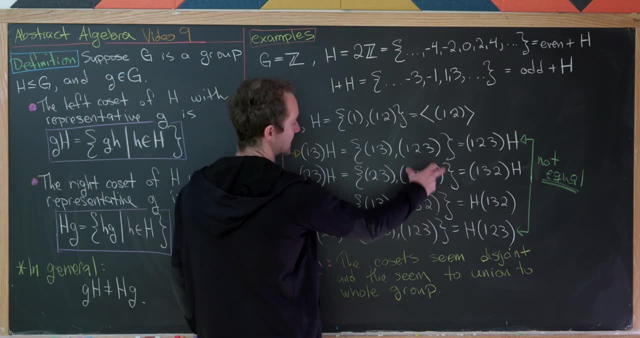 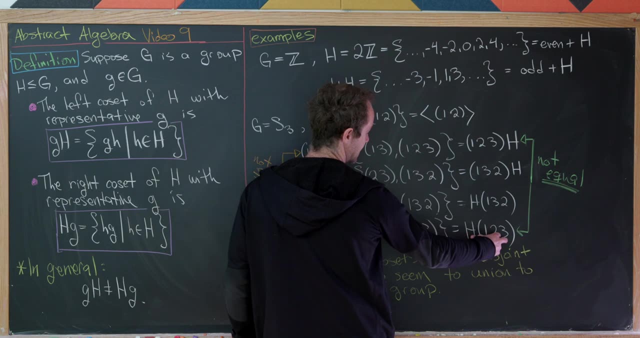 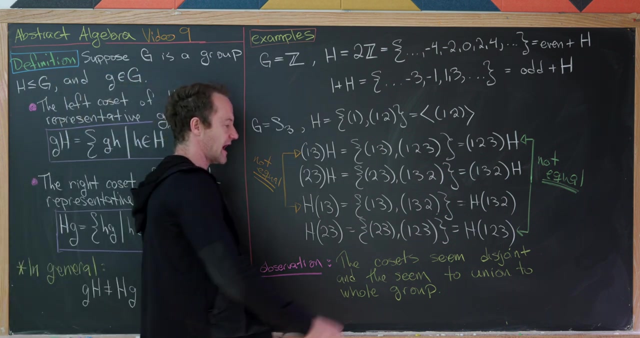 They both contain 1, 3, but they do not contain the same 3 cycle. Likewise, the right coset containing 1, 2, 3 is not equal to the left coset with representative 1, 2, 3. They have the same 3 cycle, but not the same 2 cycle. 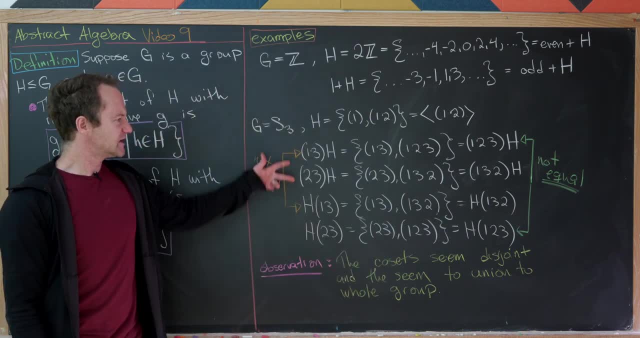 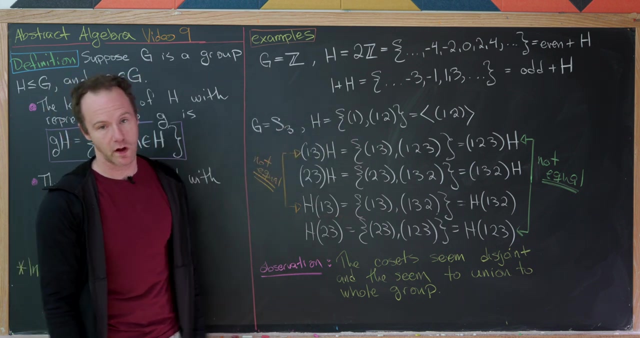 So that's interesting. But now let's just restrict our minds just to left cosets or in parallel just to right cosets. And let's notice that that group itself is both a left and a right coset where the representative is 1. And the cosets, we should maybe read this as either just the left 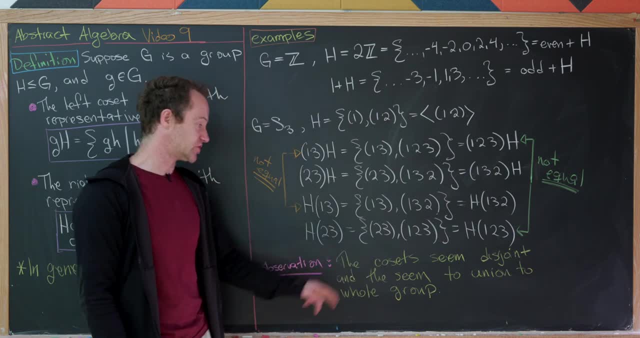 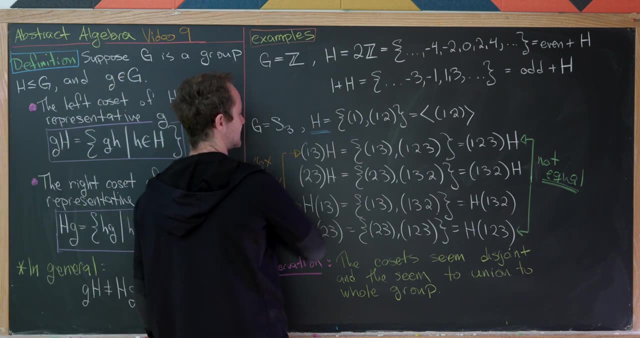 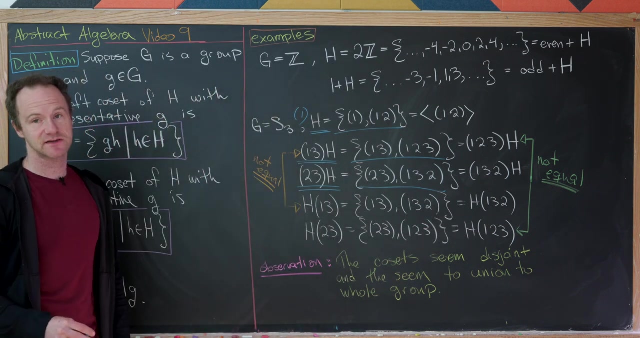 cosets or just the right cosets, are seen to be disjoint and they seem to union to the whole group. So let's look at the left cosets. We have this one right here, which nominally is attached to the identity. We have this one right here and this one right here. And notice that these sets are disjoint. They do not contain any of the same elements, but they union to the whole group. So this will be something that we prove later. Okay, 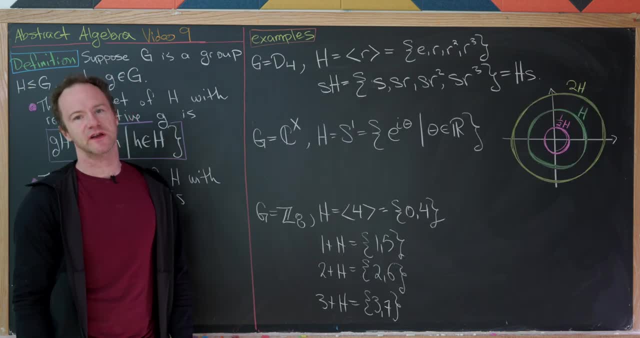 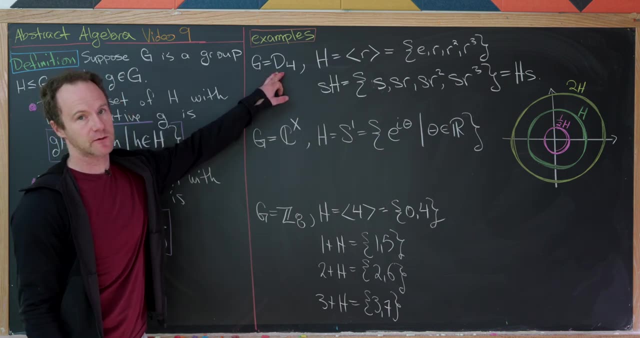 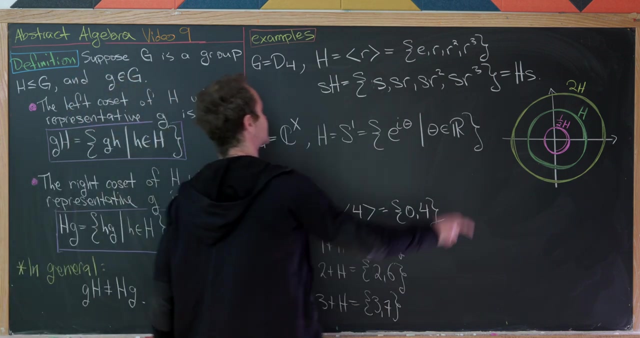 let's do a couple more examples. Here are three more examples before we start proving general results. So, let's take the group G to be D4, the symmetries of the square, and we'll take H to be the cyclic subgroup generated by R. That's all rotational symmetries. 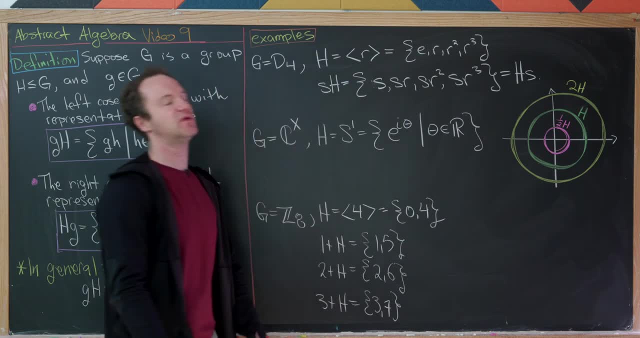 Let's recall that that will be E, R, R squared, and R cubed, because R to the fourth is back 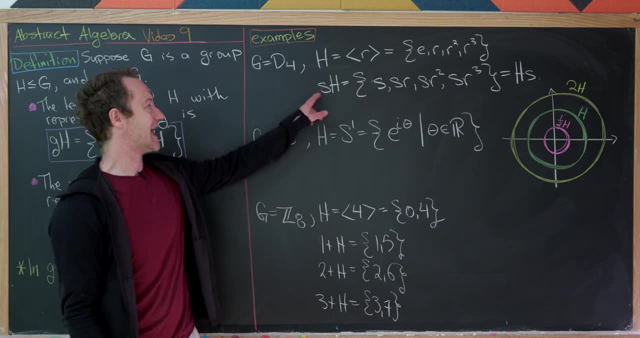 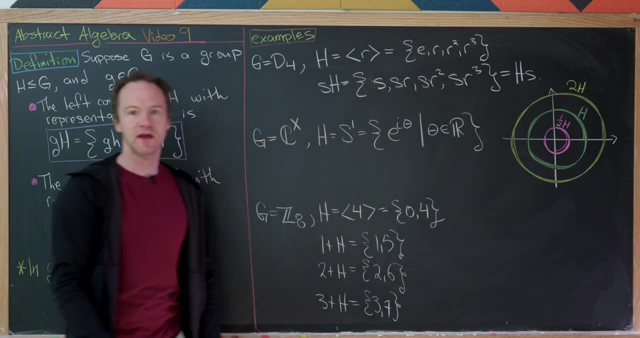 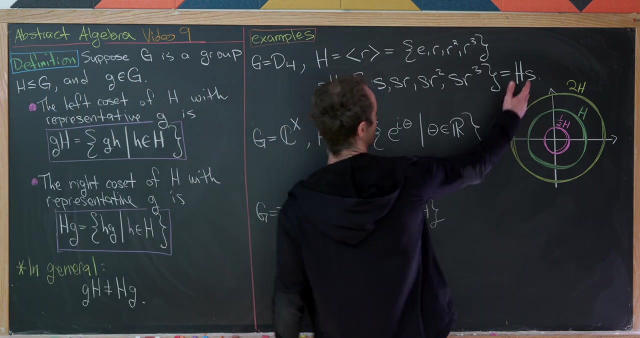 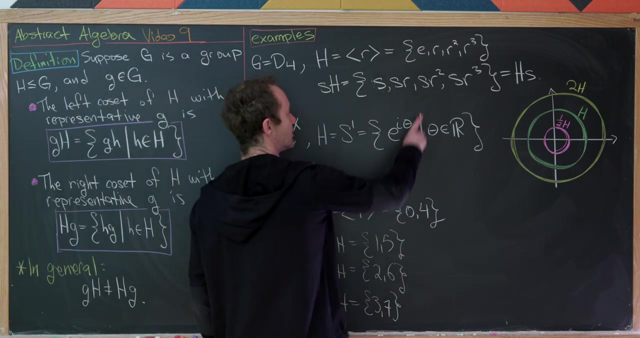 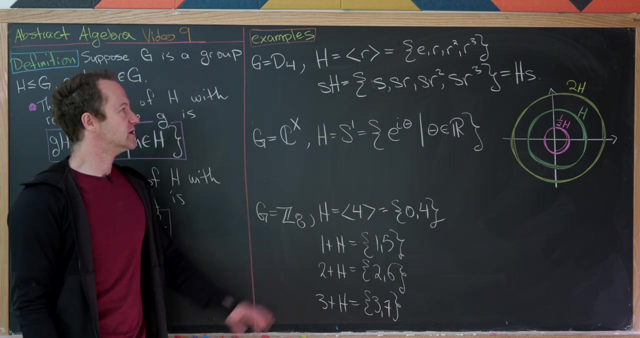 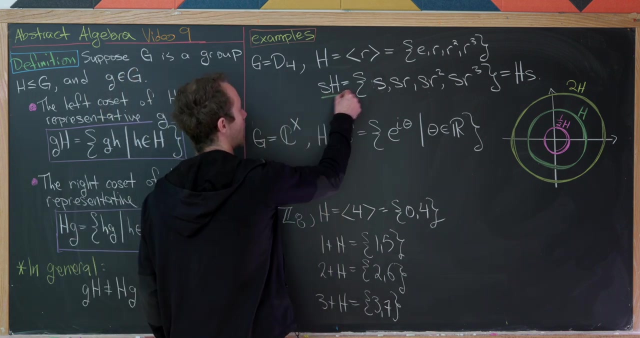 to the identity. Then let's notice that SH, that coset, will be equal to 4, and that coset will be equal to 4, and that coset will be equal to 3. And S, SR, SR squared, and SR cubed. That's all of the reflections. It does not form a subgroup though because the identity is not in there. But that's the same thing as the right coset HS. And that's simply because of the commutation rules. Notice that R squared S is the same thing as SR squared. And then after that we have like some nice commutativity like, for instance, R cubed S is the same thing as SR and R S is the same thing as SR cubed. So things get swapped around a little bit. So this is an example of a nonabelian group and a subgroup, where we in fact do have equality between the same corresponding left and right coset. 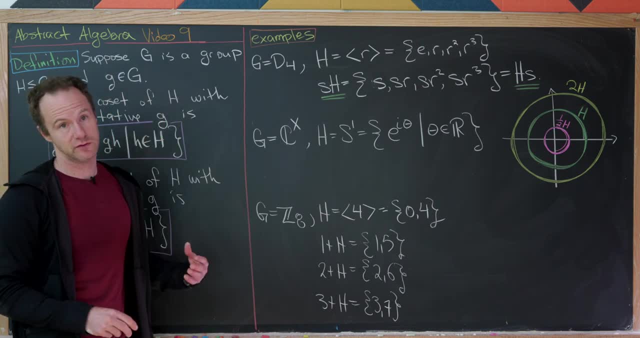 So like I said, that's going to be an important type of subgroup that leads to the same type of commutation, so it's going to be an important type of subgroup that leads to the same kind of commutation. So that's going to be an important type of commutation. So that's going to be an important type of that we'll talk about in the next video. 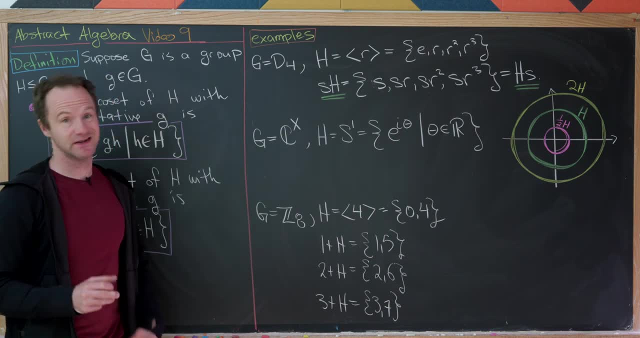 Okay, so for our next example, this is maybe one of my favorite examples because it's nice and graphical. Let's take g to be the multiplicative group 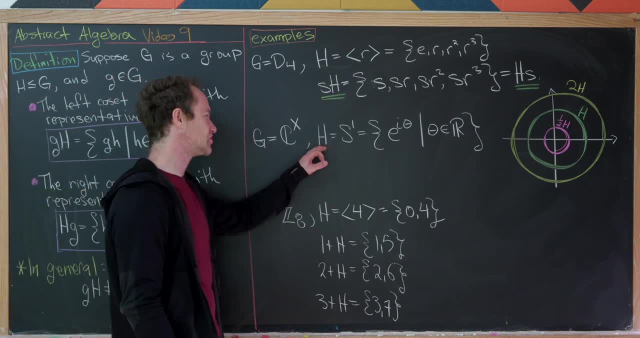 of complex numbers, and then let's take h to be the circle group. 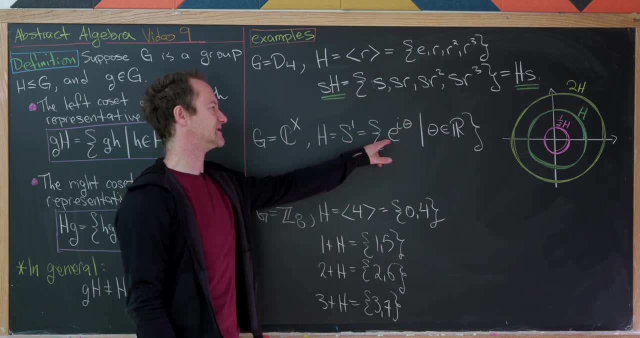 So the notation for that is s1, but let's just recall that that is everything 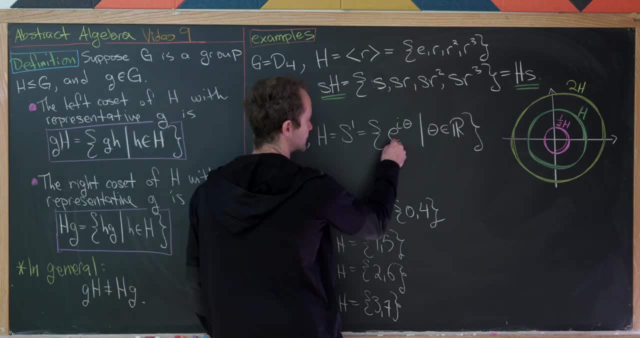 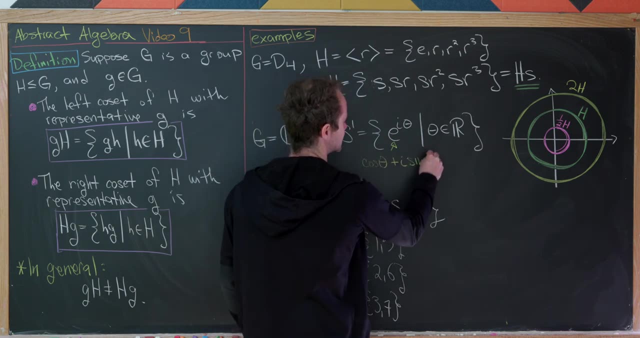 of the form e to the i theta, where theta runs through all real numbers. Recall that e to the i theta by Euler's formula is cosine theta plus i sine theta. 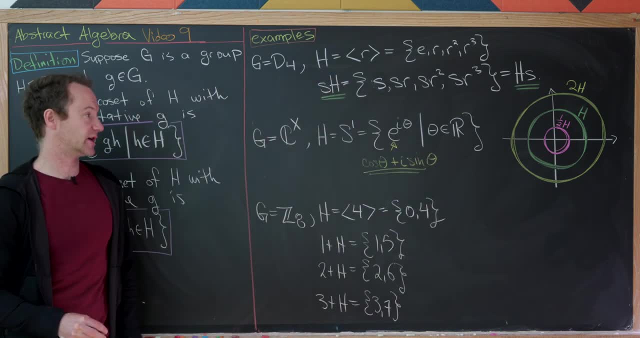 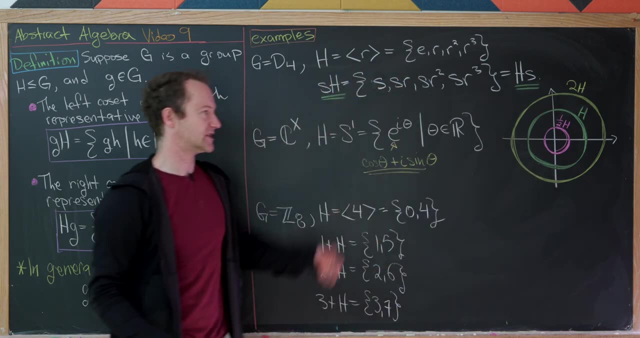 So that puts it into the complex plane. Okay, we'll notice that h itself is a circle of radius one. This is essentially the parameterization of a circle inside of the complex plane. 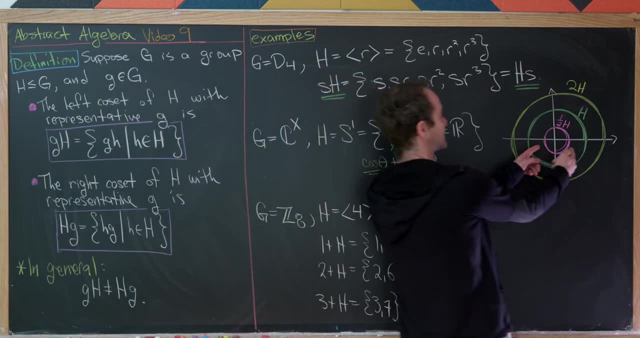 If we multiply everything in h by two, that expands the circle, and that would be the coset 2h. 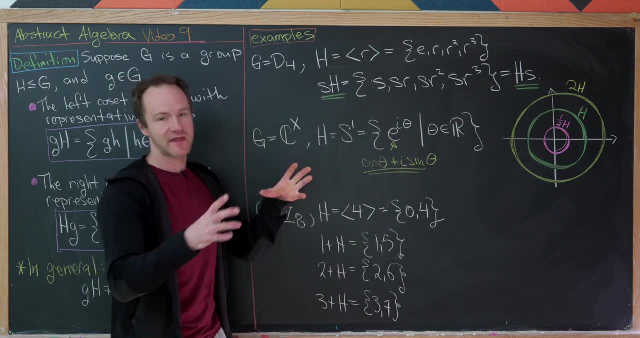 If we multiply everything in h by a half, that will contract the circle, 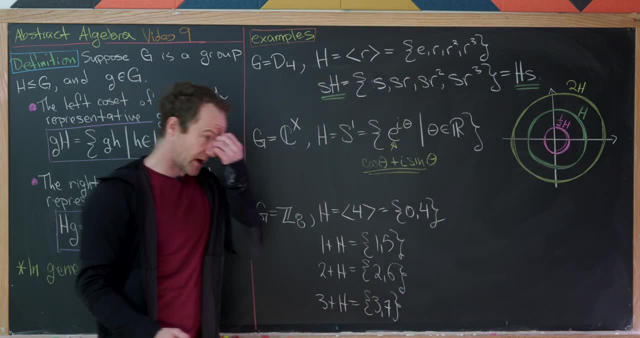 and that'll be the coset 1 half h. But actually, the number two here is not super important. 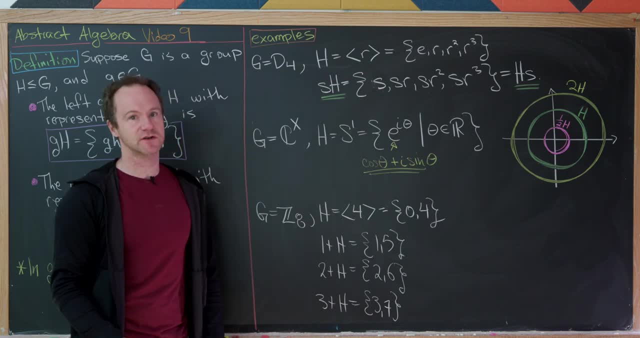 You could take any element of the complex numbers with modulus two. 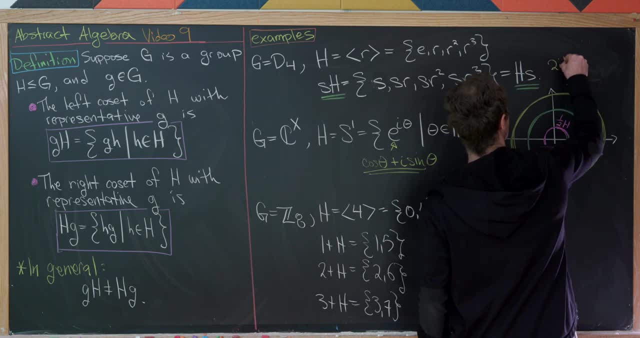 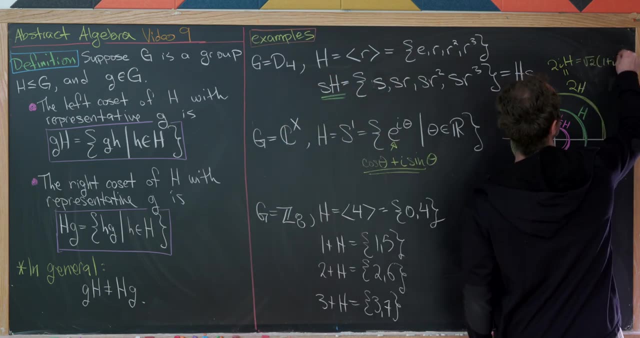 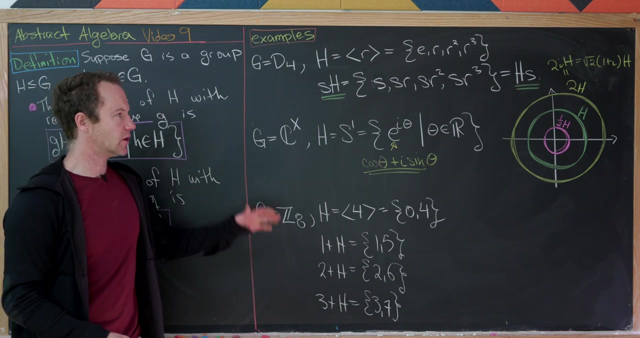 For instance, this is the same thing as two i times h. That's because two i has modulus two, and also the square root of two times one plus i times h, because that number, the square root of two times one plus i, also has modulus two. 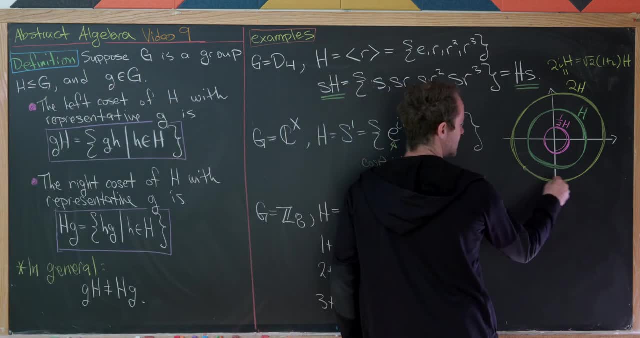 So in fact, anything along this circle could serve as a representative for the coset. 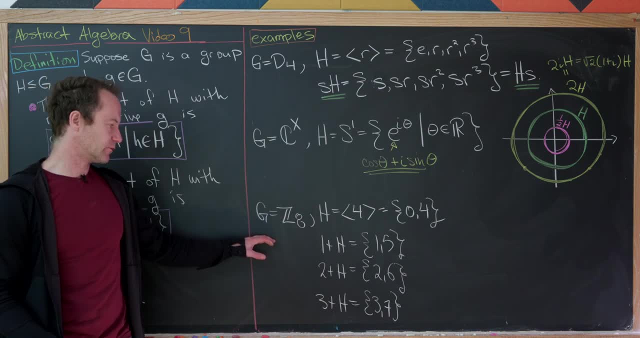 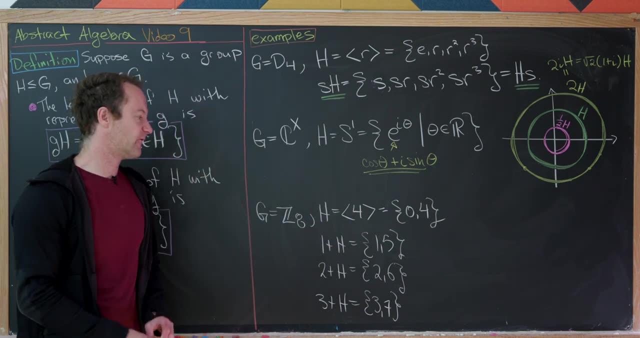 Okay, so now let's look at one last example, and that would be to take g equal to z eight, and then we'll take h to be the cyclic subgroup generated by four. 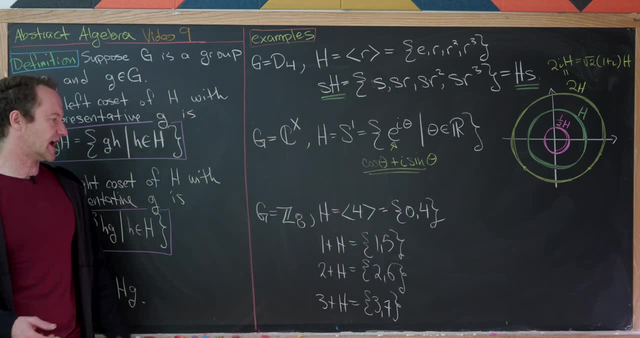 So that means it contains zero and four. Four plus four is equal to eight, which is equal to zero inside of z eight. Okay, so we have z eight. 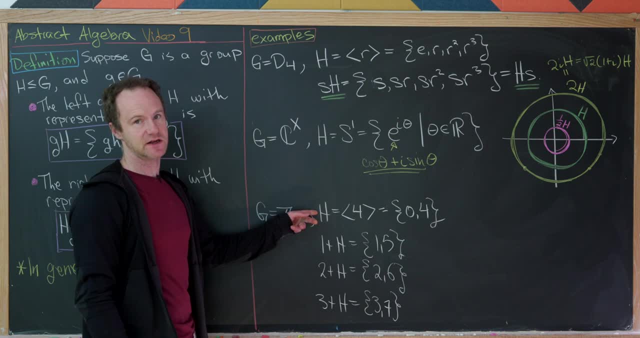 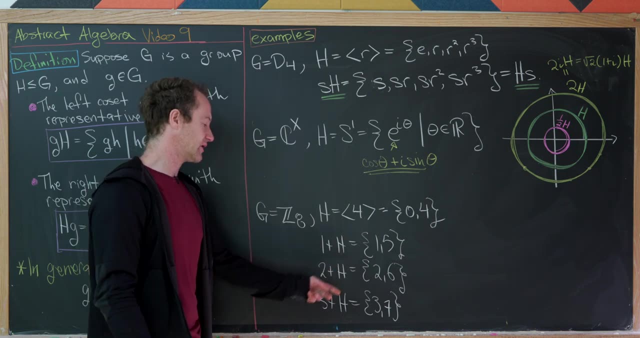 And then we've got three more cosets after the identity coset, which is the subgroup. We have 1 plus H, which is 1 and 5, 2 plus H, which is 2 and 6, 3 plus H, which is 3 and 7. 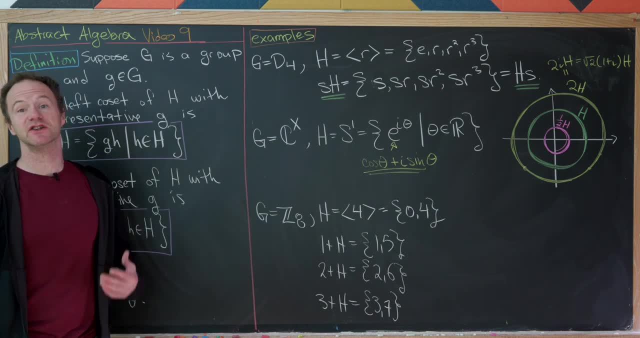 Okay, so I think this is looking good. Now let's look at a general result. 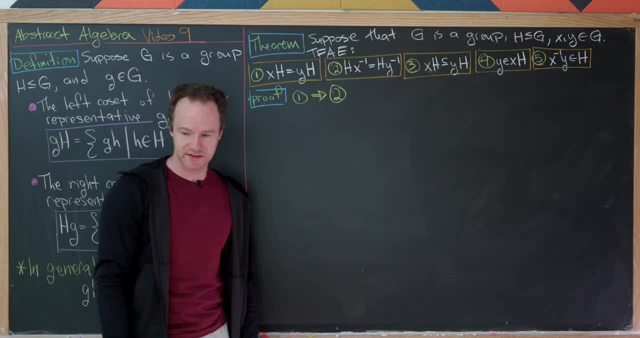 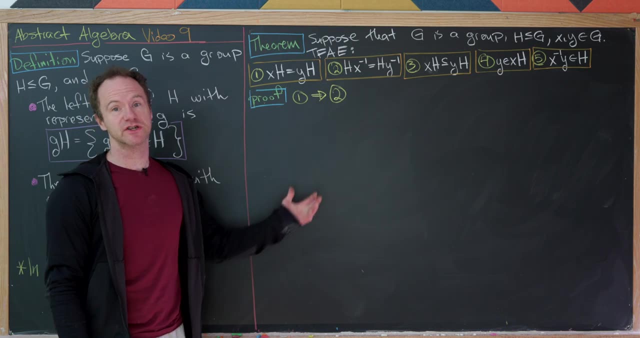 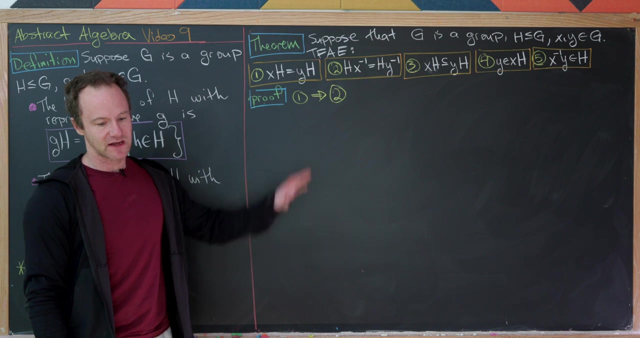 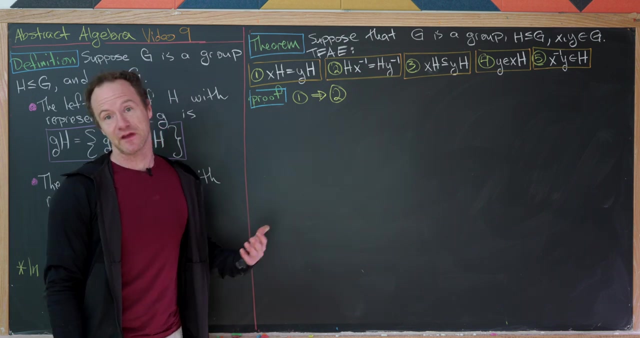 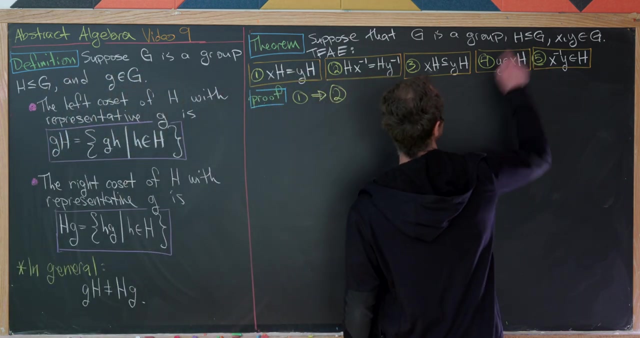 Now we've got one of the most important results involving cosets. It's so important that we'll prove it here, but I implore you to, after we prove it here, to close your notes, if you're taking notes, and then try to prove it on your own without rewatching the video or taking notes. It's really important to kinda understand the tricks that we'll use in this proof. So like I said, this is a proof that maybe all math majors should be able to just come up with after they've taken an abstract algebra class. Okay, so let's see what we have. Let's suppose that G is a group, H is a subgroup of G. 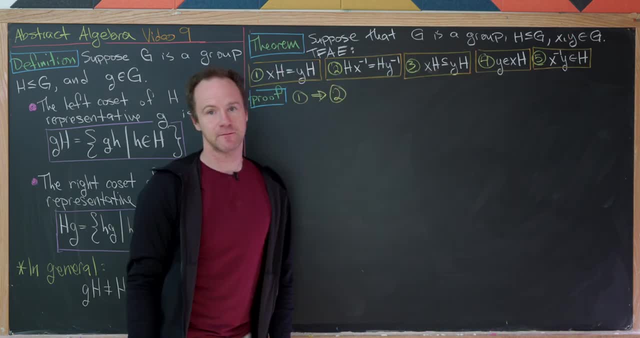 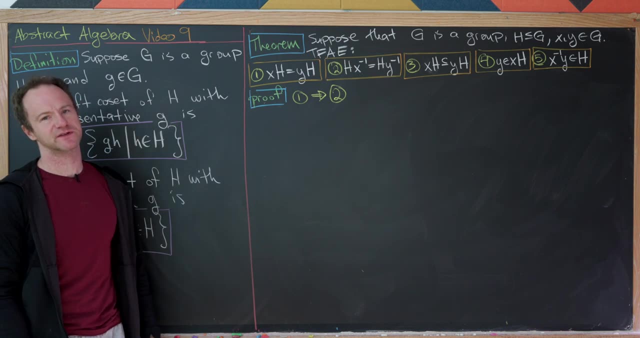 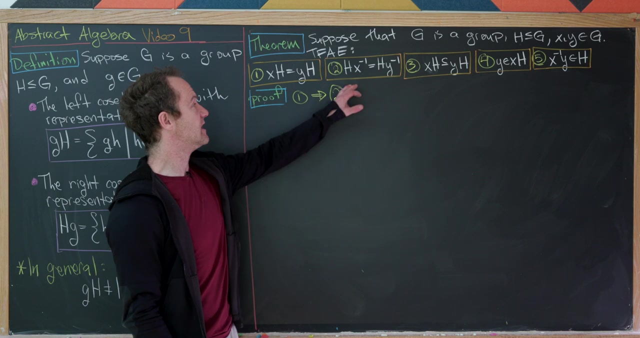 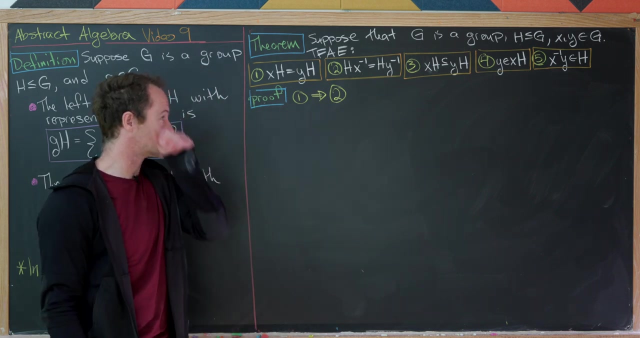 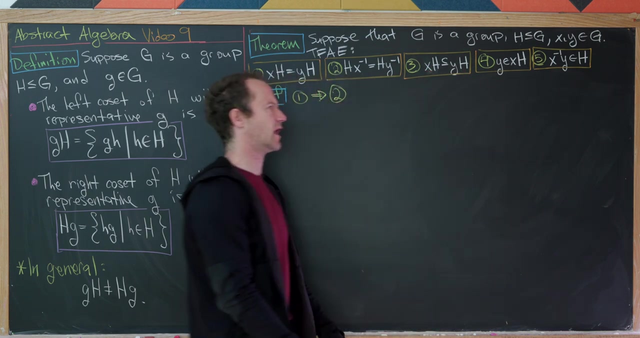 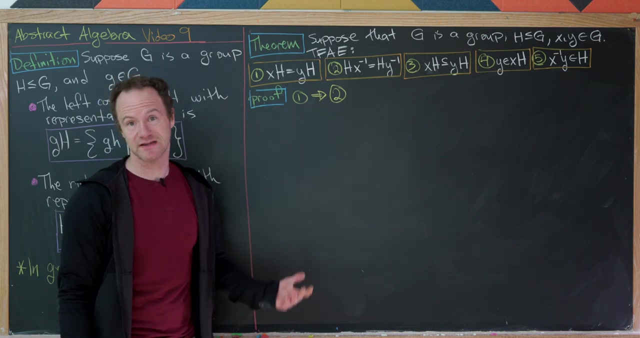 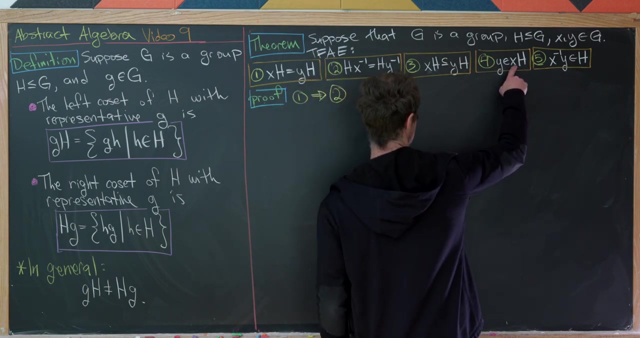 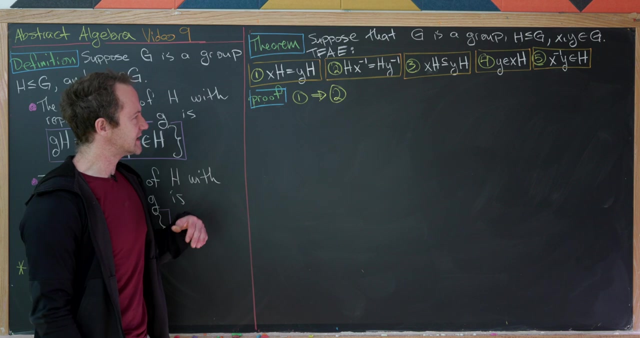 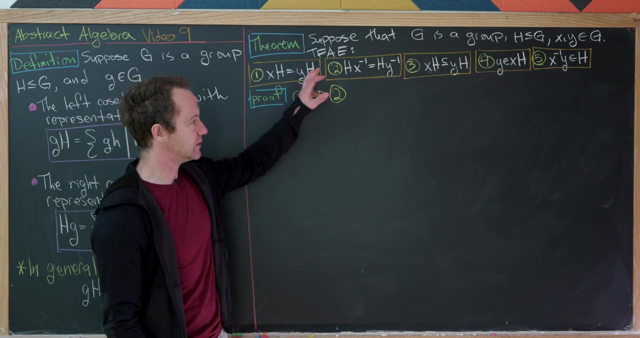 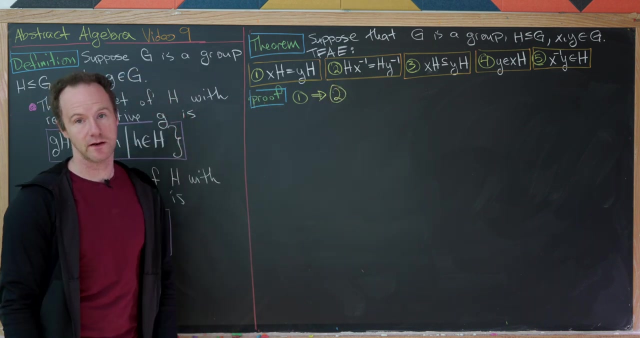 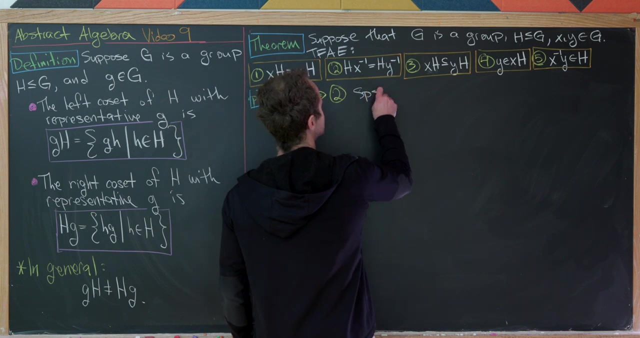 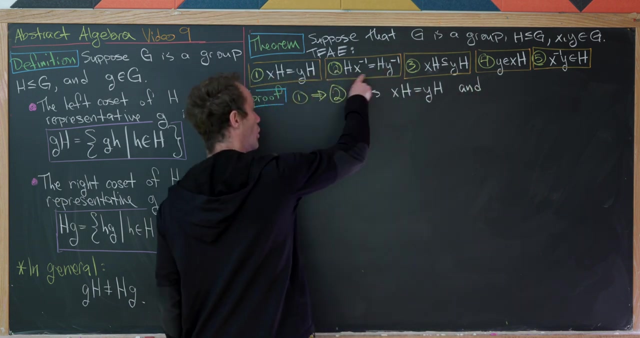 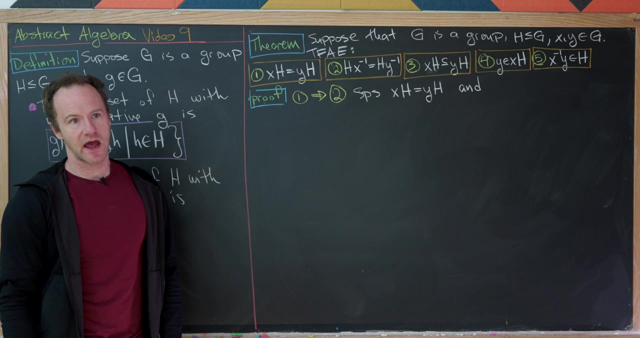 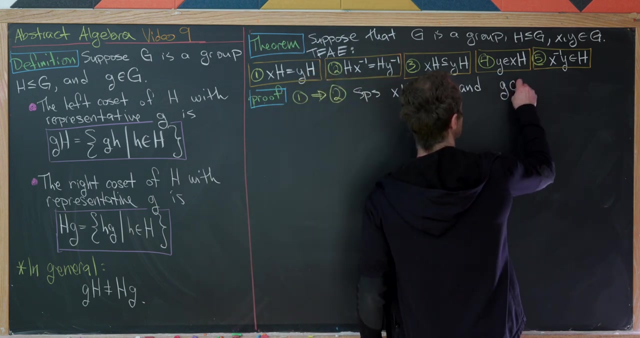 And then H is the subgroup of G. x and y are elements of g. And what this theorem is about is when cosets are equal. So we saw that cosets with different representatives were equal already. Okay, so then we have the following five statements are equivalent. So the first is the coset xh is equal to the coset yh. And then next is the right coset hx inverse is equal to the right coset hy inverse. Next is that the coset xh is a subset of the coset yh. So that's on its face pretty interesting that that is equivalent to equality. We have containment is equivalent to equality. Next is that y is an element of the coset xh. And finally we have xx. inverse y is an element of h. Okay so let's get to the proof and we'll do this proof with a looping action. We'll prove 1 implies 2, 2 implies 3, 3 implies 4, 4 implies 5, and then finally 5 implies 1. And that will show that they're all equivalent. Okay so anyway let's get to 1 implies 2. So let's suppose that xh is equal to yh and then our goal is to show that these right cosets are equal. So hx inverse is equal to hy inverse. And how do we show two sets are equal? Well by double set containment. So that means we need to take an element g inside of the left one and show that it's inside of the right one. So we've got g inside of the right one. And then we need to 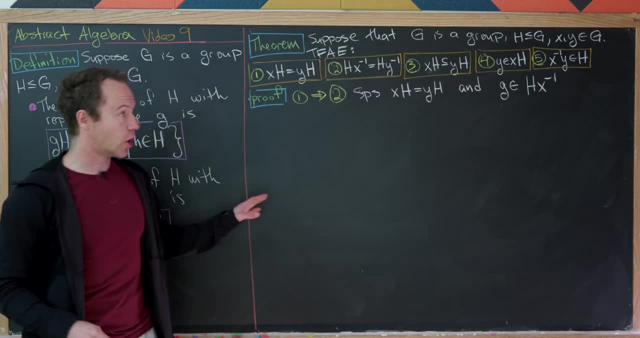 hx inverse. And then our goal is to get g inside of hy inverse. That would show the subset 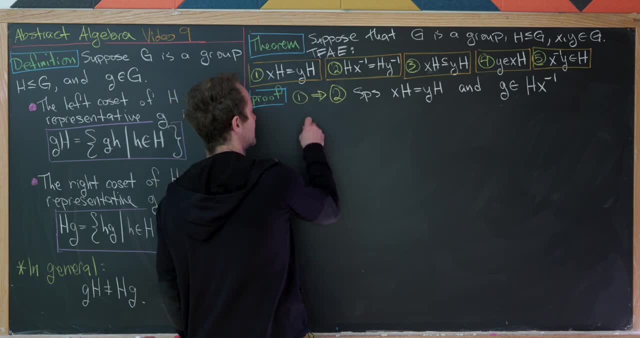 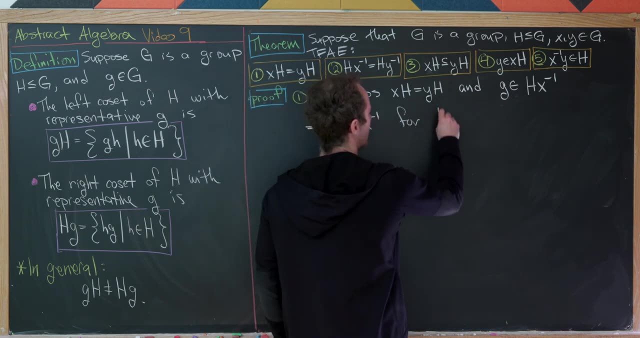 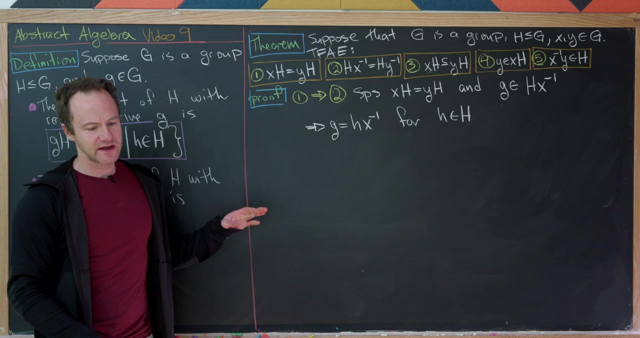 relationship. Okay so anyway let's get to it. This tells us that g is equal to little h times x inverse for a little h inside of h. Okay but now what we'd like to do from here is somehow get the 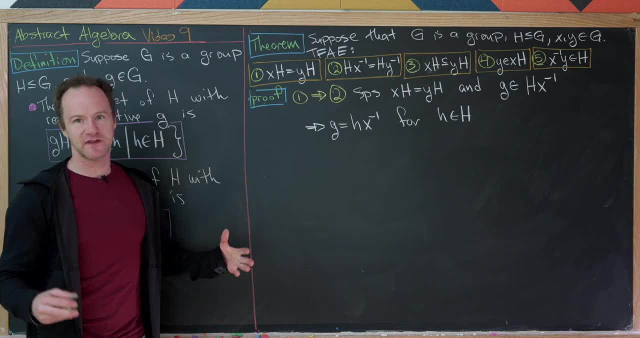 element of h to the right. So we're going to get g inside of hx inverse. And then our goal is to get g inside of hy inverse. And then our goal is to get g inside of hy inverse. And then our goal is to right. And we want to get the element of h to the right because then we can use this fact that we 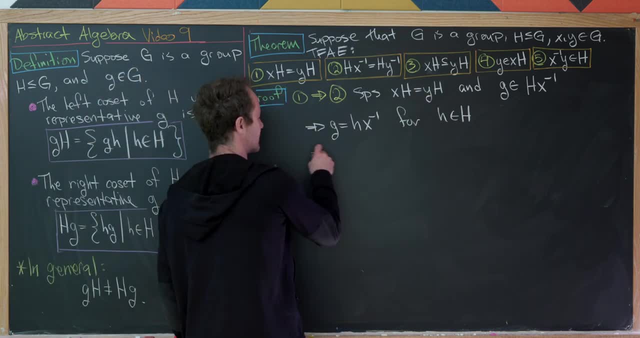 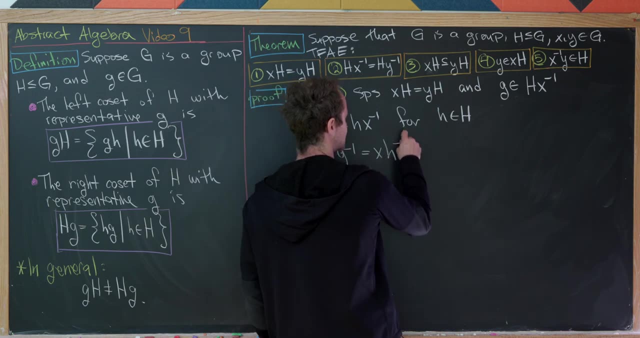 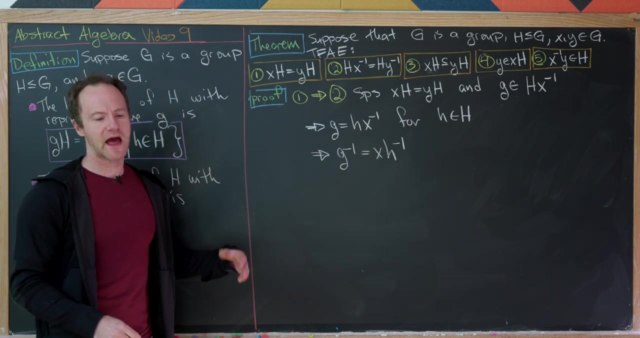 know about left cosets. So let's invert this equation. So that tells us that g inverse equals x times h inverse. Remember we applied the shoes and socks theorem to this right side. That rule about how inverses affect the order of multiplication. Okay but now let's notice that this is 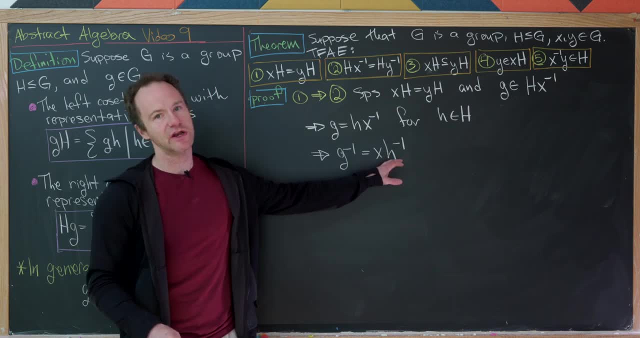 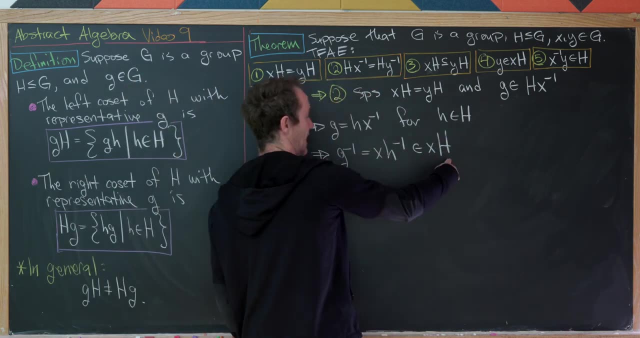 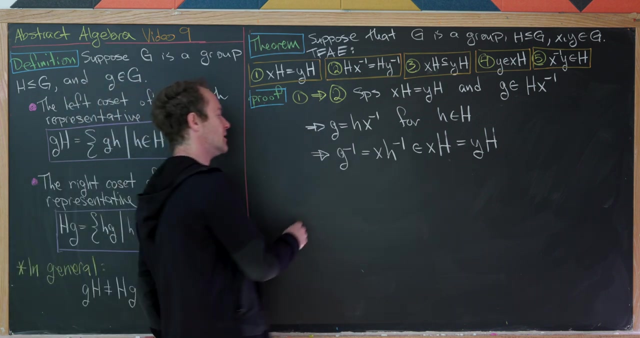 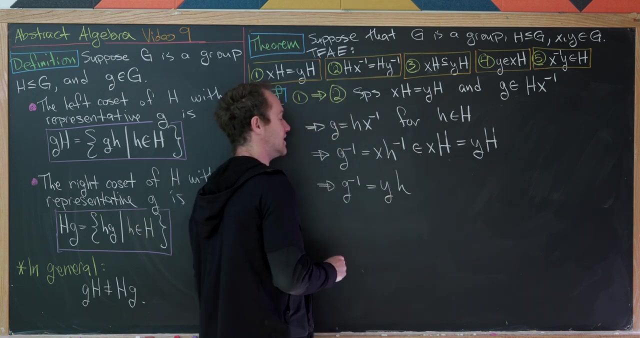 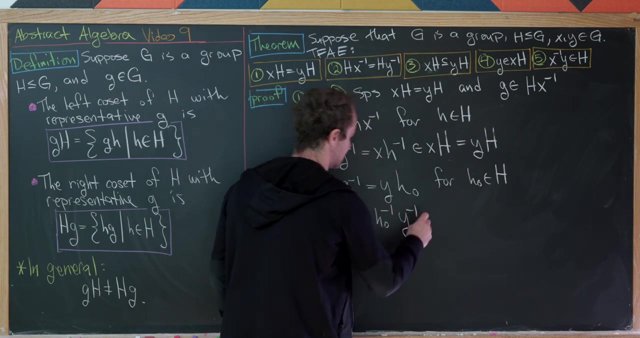 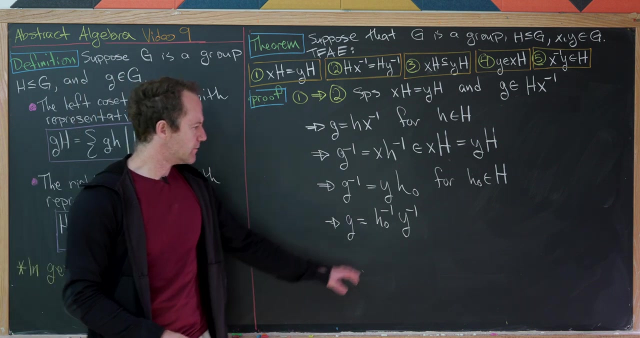 equal to x times something in h. We know h inverse is in h because h is a subgroup. So this is inside of the coset xh. But that coset xh is equal to the coset yh by our assumption. But what does that mean? That means that little g inverse is equal to y times a new h. Maybe we'll call this h0 for h0 inside of h. That's what it means to be inside that left coset yh. But now we'd like to invert this again and see what that leaves us with. So let's invert this and we'll get h0 inverse y inverse over there on the right hand side. That's because g inverse inverse is just g. Oh but now 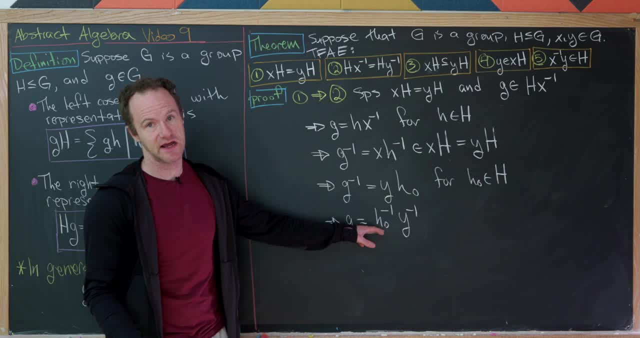 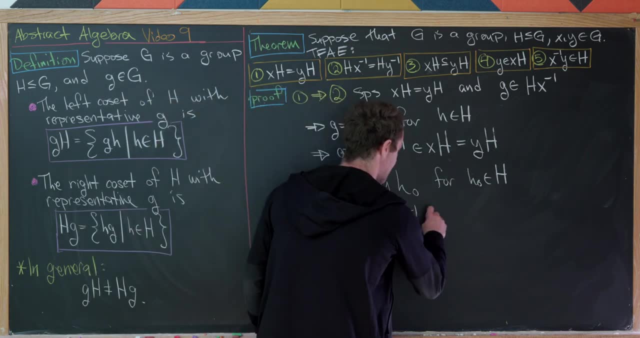 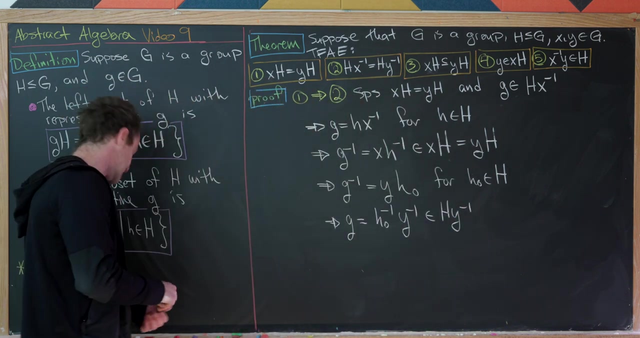 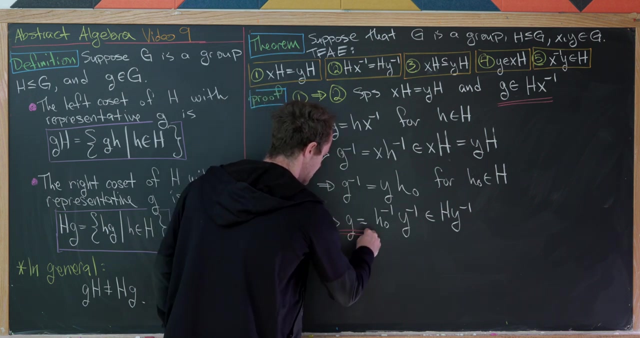 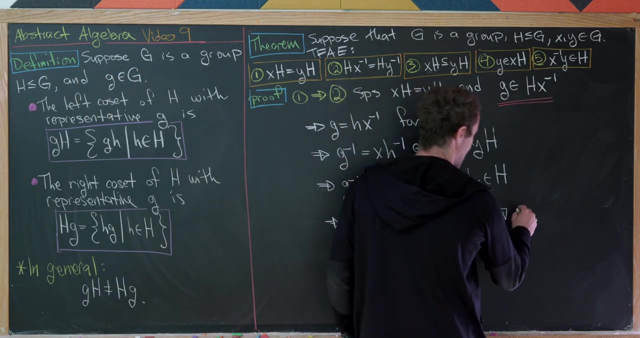 this is an element from h. Remember h0 is in h. So h0 inverse is in h because h is a subgroup. This is an element of h times y inverse. But that is the entry fee to be inside of h y inverse. Okay so let's see what we got. We started here with g is inside of hx inverse and we ended here with g is inside of hy inverse. So those red underlines imply that hx inverse is a subset 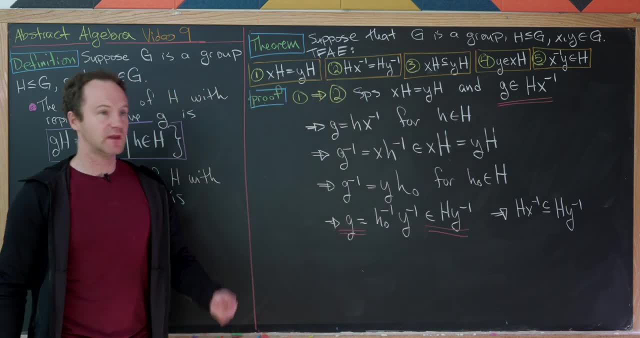 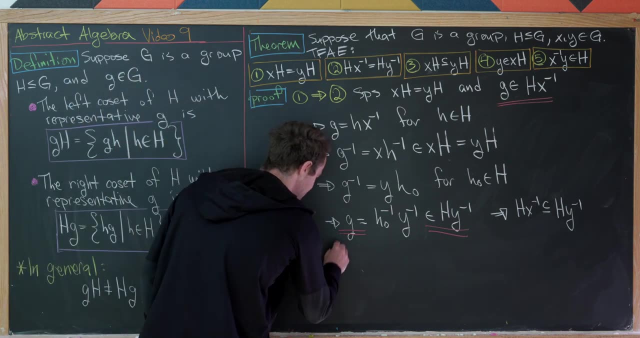 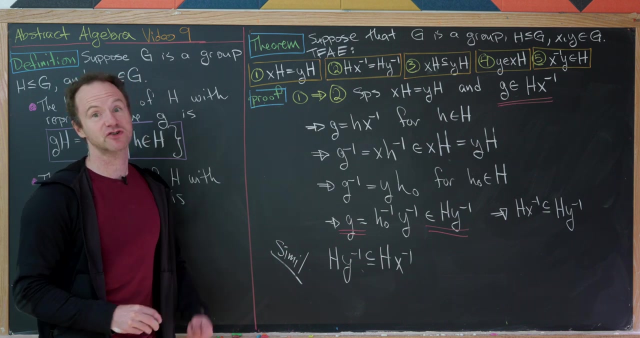 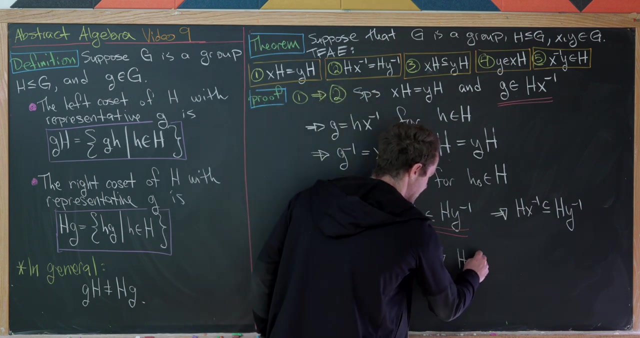 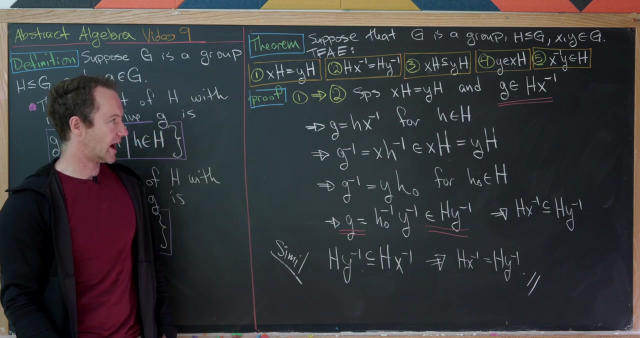 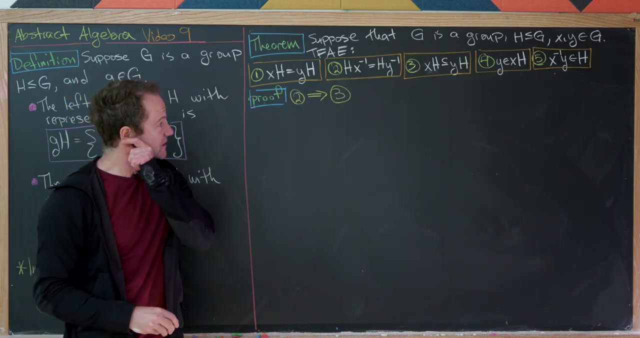 of hy inverse. Okay then we also have to show that hy inverse is a subset of hx inverse. But I'll leave that for you because it is exactly similar. So similarly hy inverse is a subset of hx inverse. And that's essentially because x and y are playing symmetric roles in this setup. So now these two things together do give us equality of these right cosets. So we've got hx inverse is equal to a hy inverse but that's exactly this 2. So that proves the statement 1 implies 2. And now let's move on to 2 implies 3. 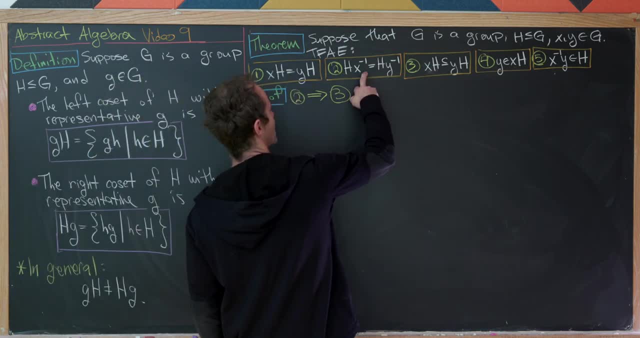 So let's see. We'll need to start with this statement right here and 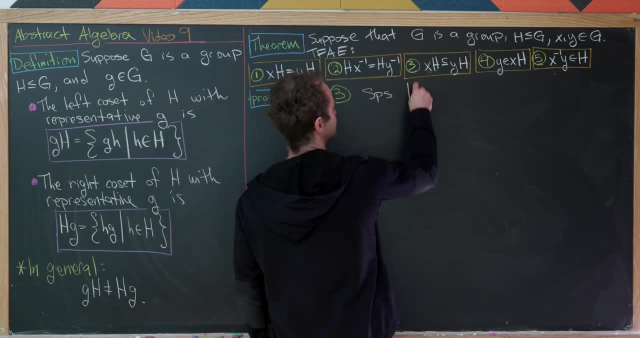 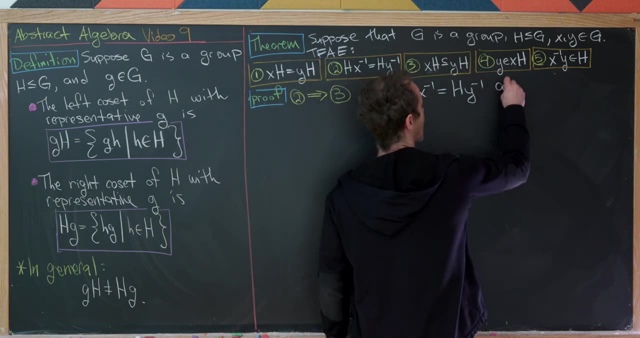 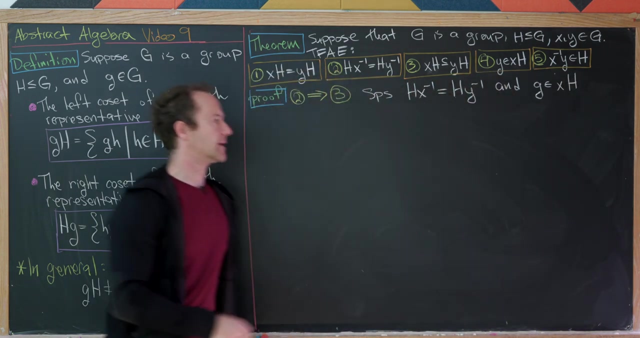 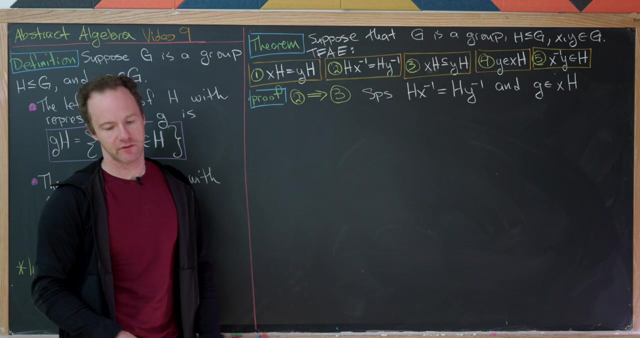 end with this statement right here. So let's suppose that hx inverse is equal to Y inverse as right cosets, and that we have a little g inside of XH. Okay, and then our goal is to get that little g inside of YH, and that'll prove this subset relationship that we need. 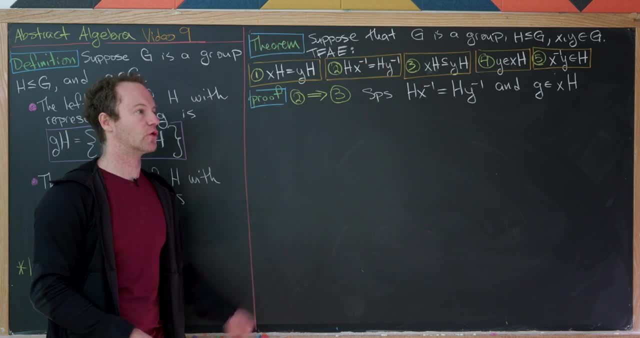 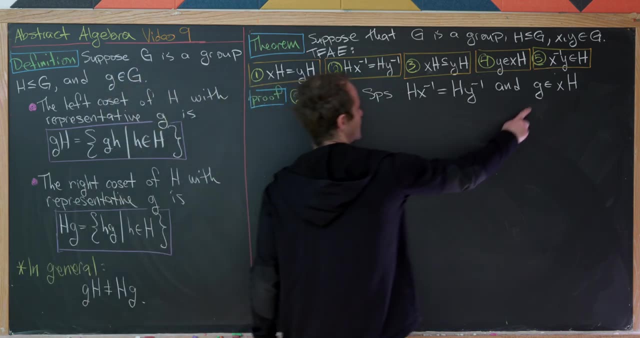 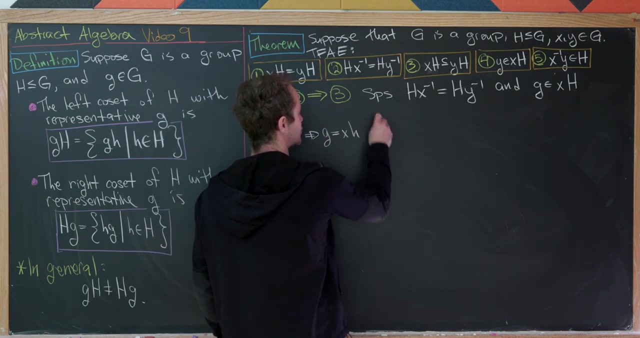 But this is going to be essentially the same as we did before, except there's no reverse direction to do. That's because we just need set containment in this case. Okay, so what does it mean for little g to be in XH? Well, that means that little g is equal to XH for some little h inside of H. 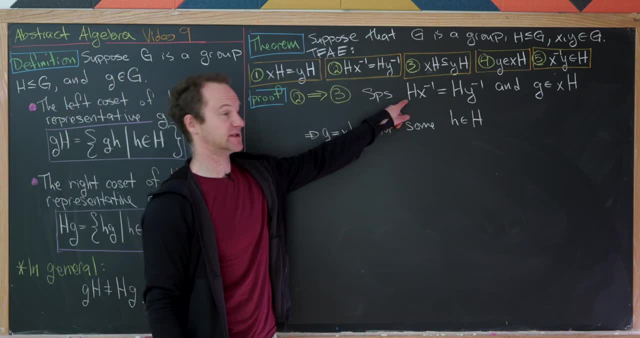 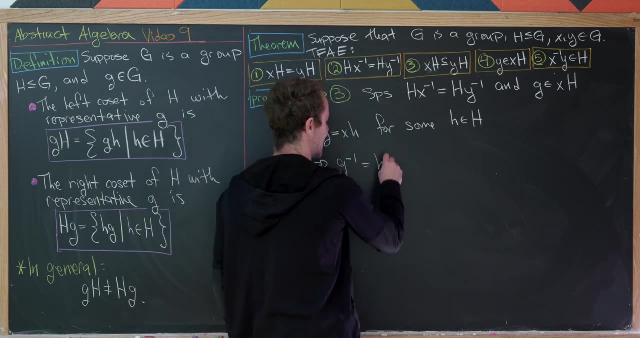 But now we'd like to get X inverse involved because we want to use this given. So let's invert this thing. That'll give us g inverse equals H inverse X inverse, but that's the shape of something inside of HX inverse. 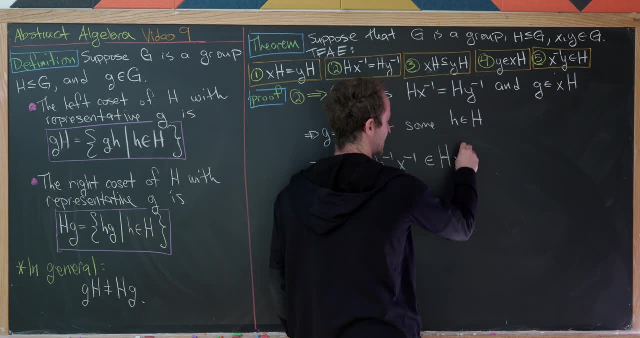 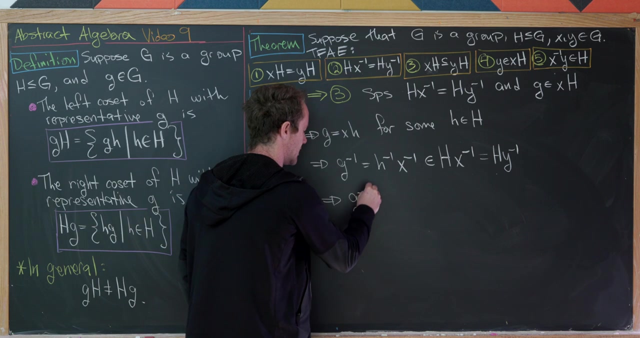 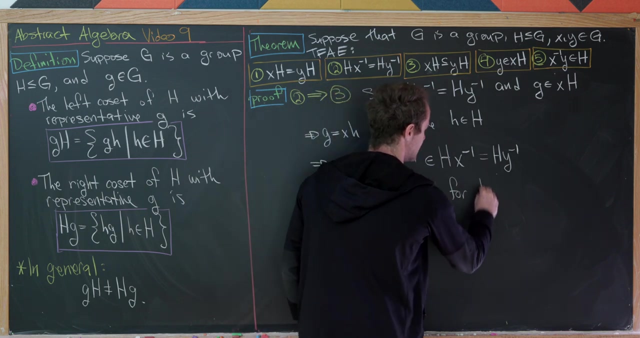 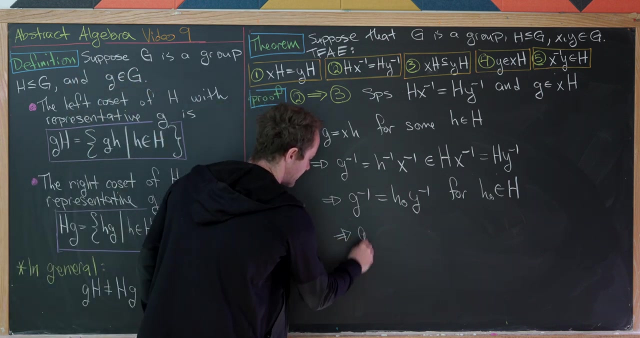 So that means this is inside of the right coset HX inverse. But by our assumption, that's equal to the right coset HY inverse. But g inverse being inside of that coset means that we can write it in the following form. We have g inverse is equal to H naught times Y inverse for some H naught in H. Now we're going to invert this thing, and essentially, this is going to be done. So inverting, we'll get g is equal to Y times H naught inverse. 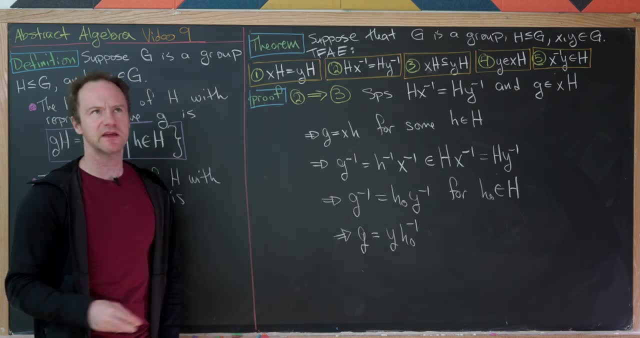 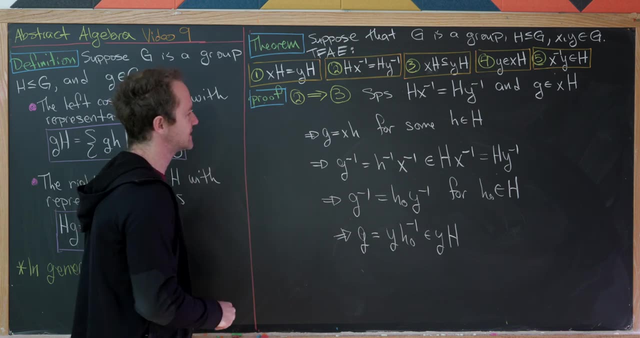 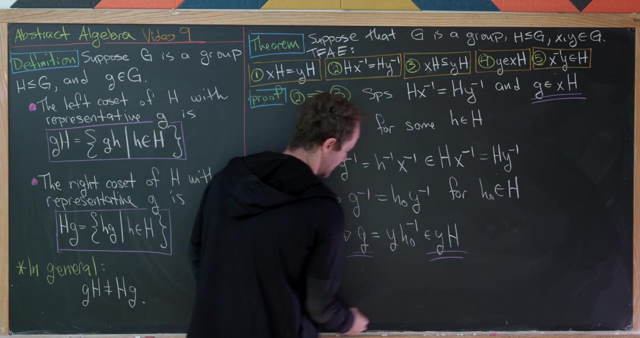 But that's Y times something in H, again, because H is a subgroup. So this is inside of the left coset YH. Okay, so let's see. We started right here with g is in XH, and we ended right here with g is in YH. So that starting and ending point tells 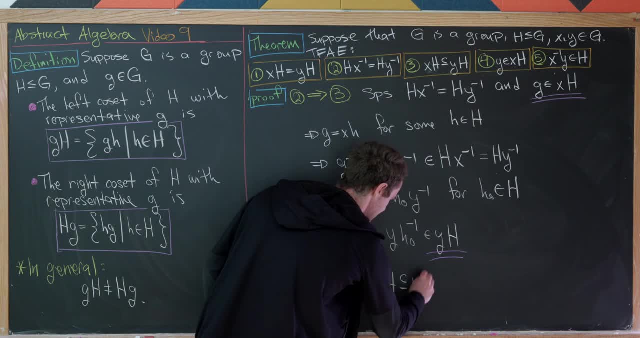 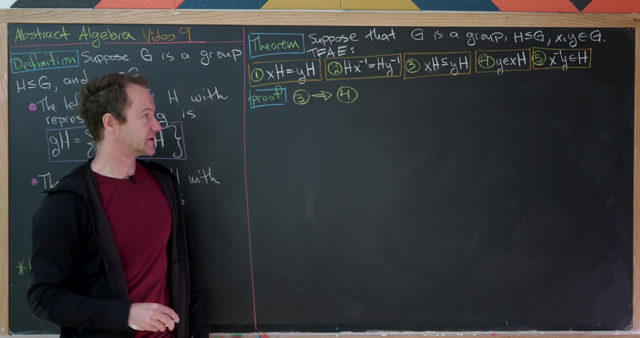 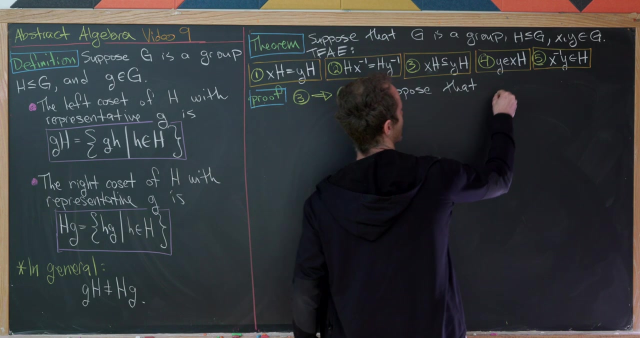 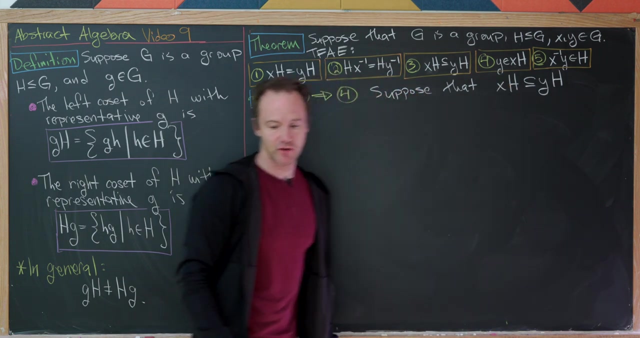 us that XH is a subset of YH. But that's exactly where we needed to go for this number three. And now we're ready for three implies four. So let's suppose that we have this set 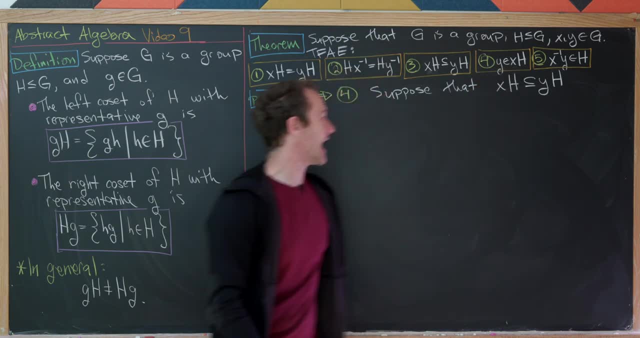 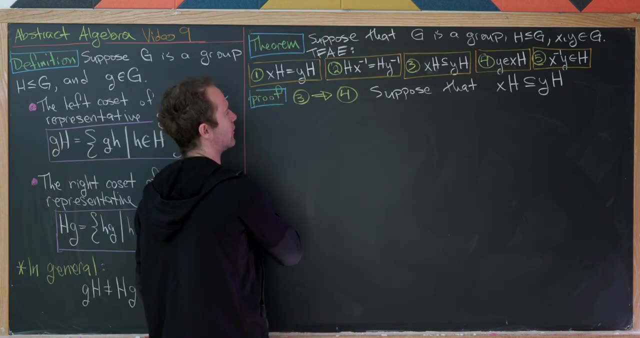 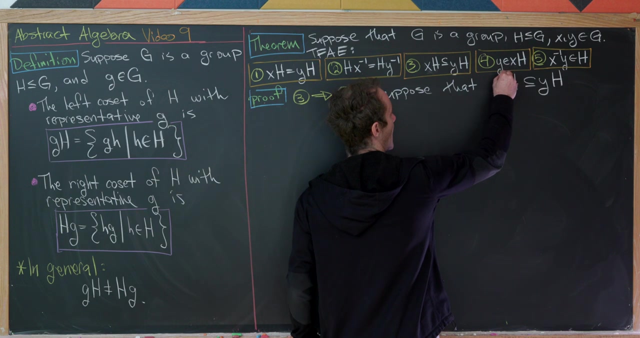 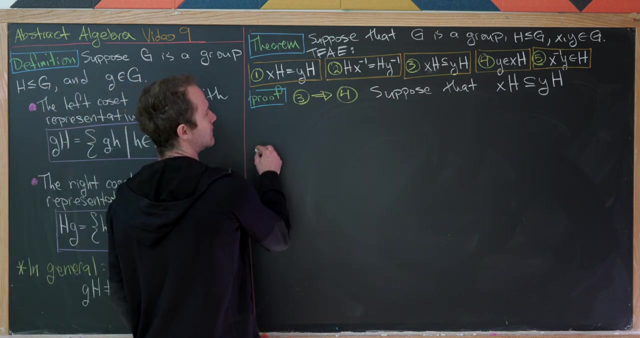 Y is inside of X times H. But let's see. We can't immediately do this the way that we did before because we had subset relations in these previous steps. We want to show that an element Y is inside of this coset XH. So that means we've got to do something different here. Maybe the most important starting point will be to notice that since we're going to 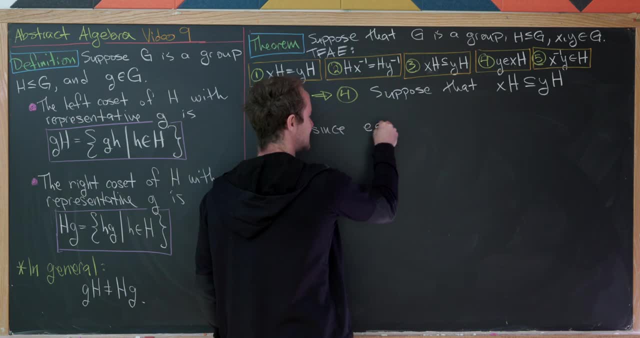 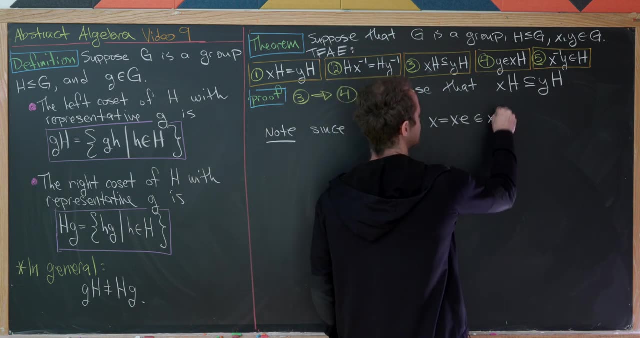 have elements H is a subgroup, we have the identity is inside of H, which tells us that X, which is equal to X times the identity, is inside of the coset XH. So we're guaranteed 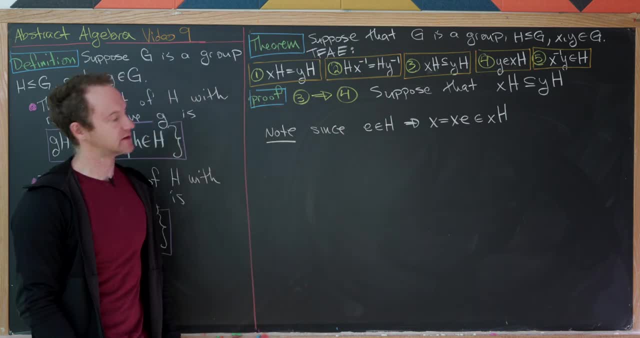 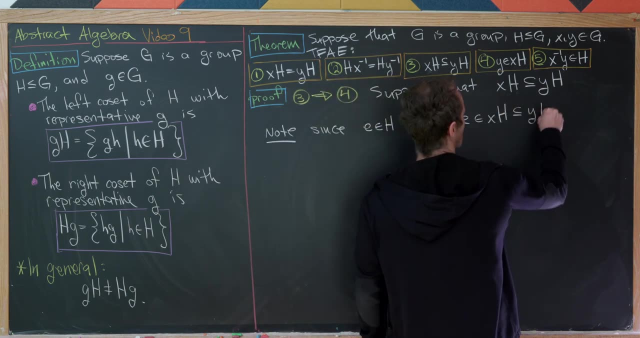 to have the element X inside of its coset. Okay, but now we assumed that XH was a subset of YH. So what does that mean? Well, following this from the left, 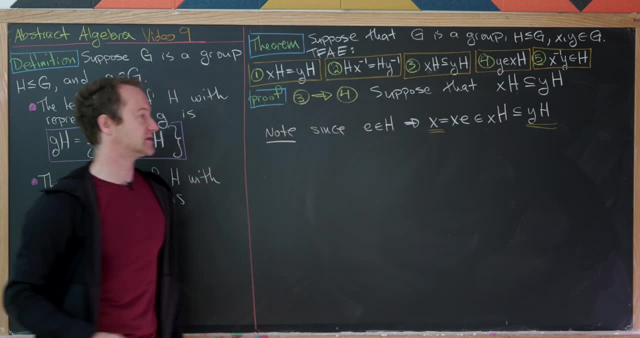 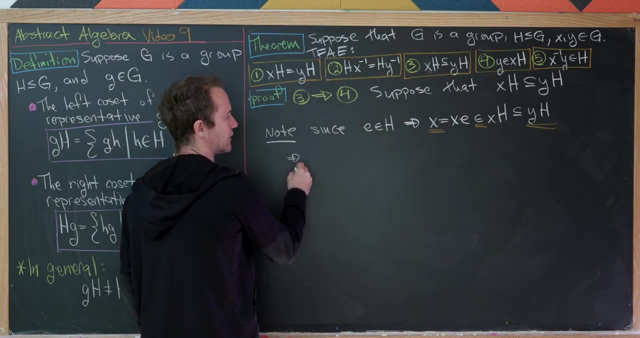 to the right, we see that X is an element of YH. Let's recall we have that element right there. What does that mean? That means that we can rewrite X as little y times H for some 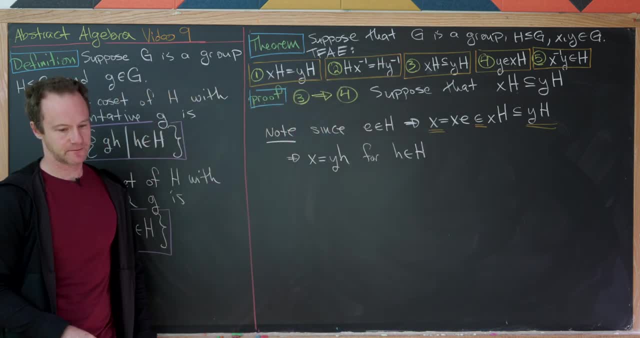 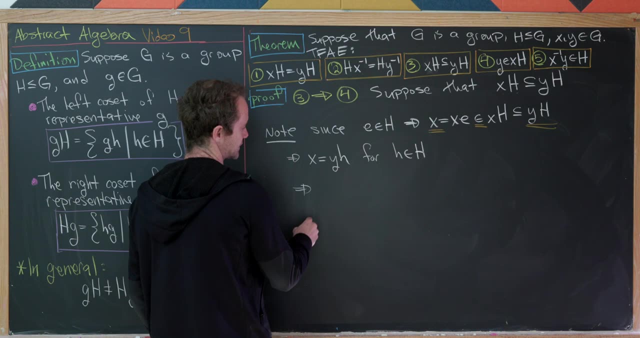 little h in H. That's what it means to be in that coset. And now from here we'll just right multiply by H inverse. Now right multiplying by H inverse will give us, let's see, will 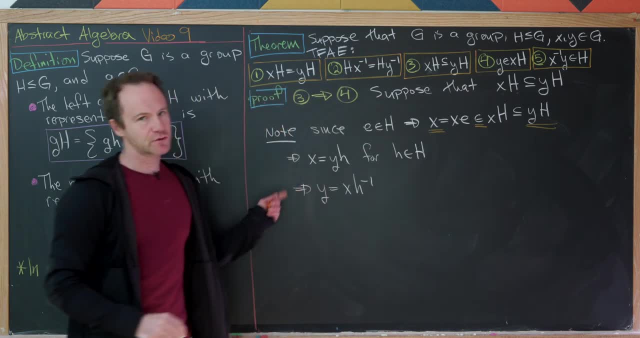 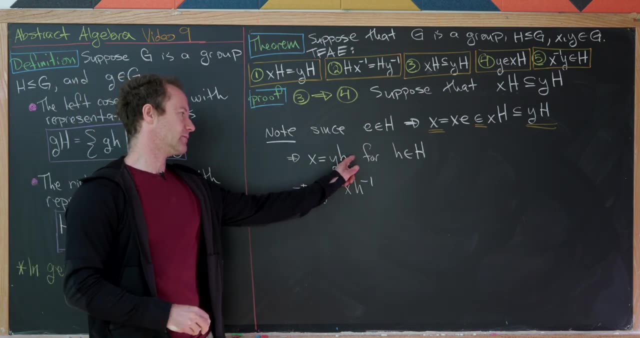 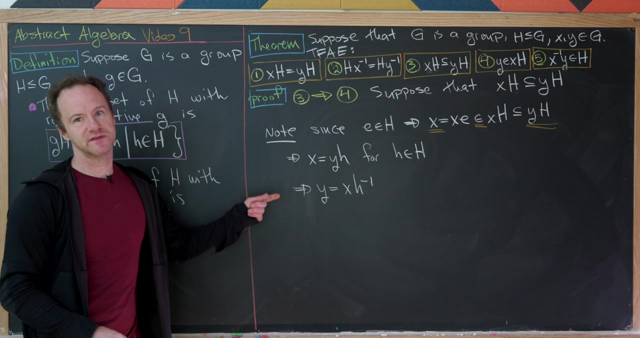 be y equals XH inverse. I swapped the order of the equality there, but that's okay because equality is symmetric. So just to reiterate, I right multiplied by H inverse, and that's going to kill the H here and give us XH inverse. But since H is a subgroup, H inverse is an 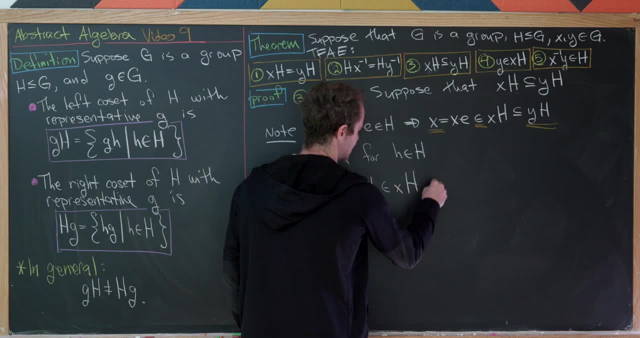 H, so that means this is an element of XH, that coset. But that's exactly where we wanted to end up with for this number 4. 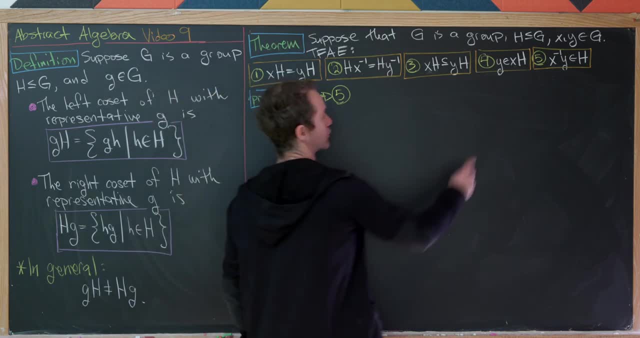 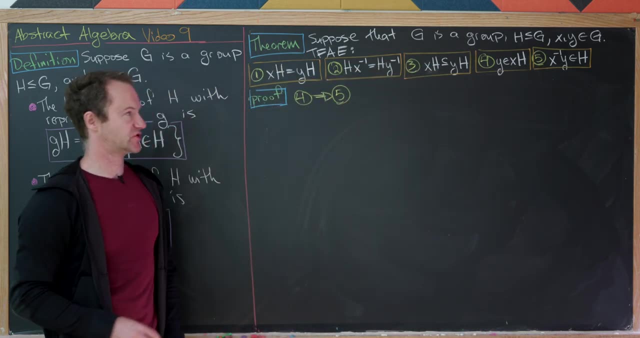 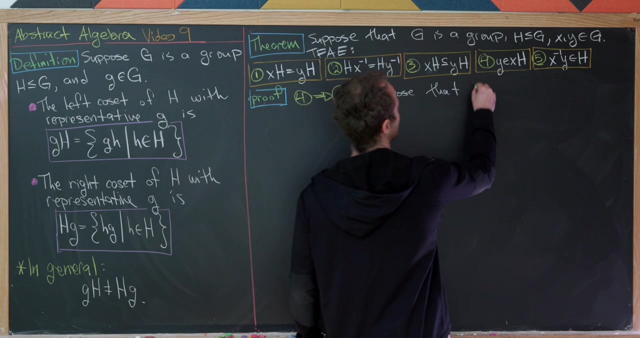 Now, moving on to number 4, we want to start with Y is an element of XH and prove that X inverse H is an element of H. This is another pretty quick one. So let's suppose that we have our assumption Y is an element of XH, but that means that Y is equal to X times 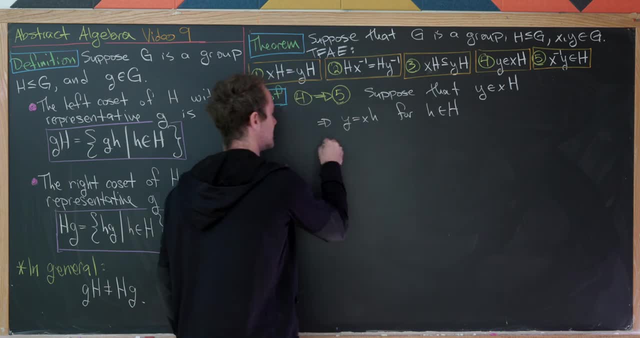 little h for some little h in H. Right multiply by X inverse on both sides, and that's going to give us X inverse times Y is equal to H. But H was inside of H. So now we have X inverse times Y inside of H as needed. 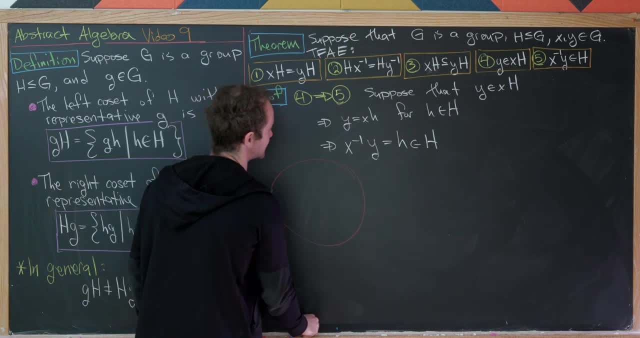 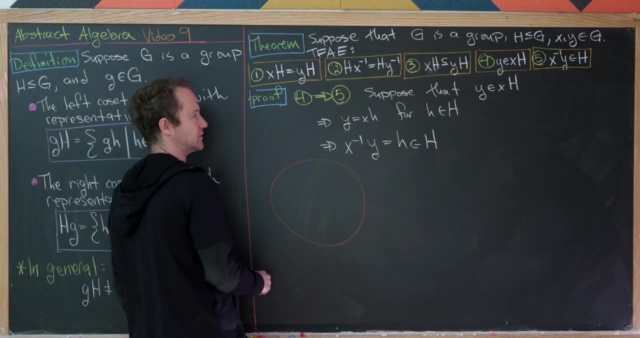 Now in this case, before moving on to the next and last bit, I'd like to prove that there are some equivalent statements here that are also fairly useful. Like this is the same thing as X, Y, H. 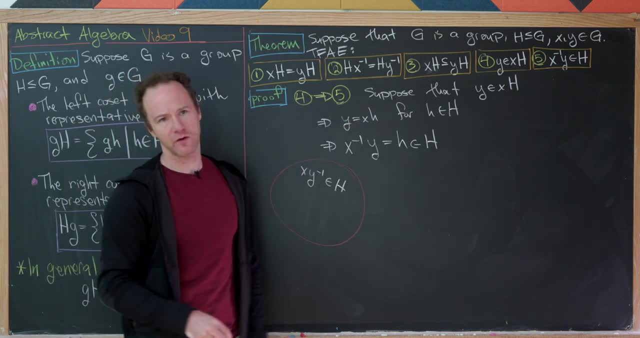 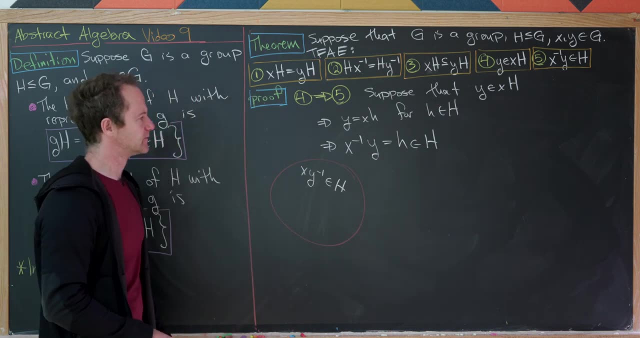 Y inverse is in H. And that doesn't follow from number 4, but through like an equivalent symmetric argument, we can land at something like this. 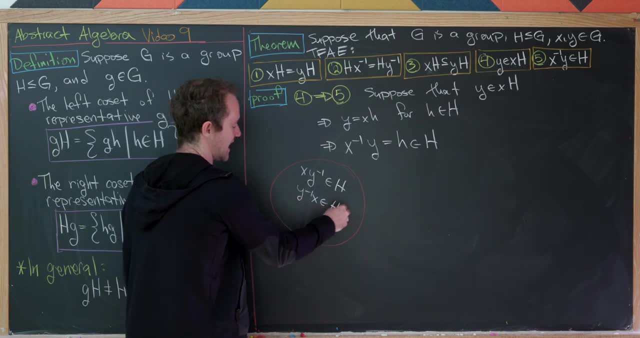 Also we could maybe see immediately that Y inverse X is in H, and a number of different things. 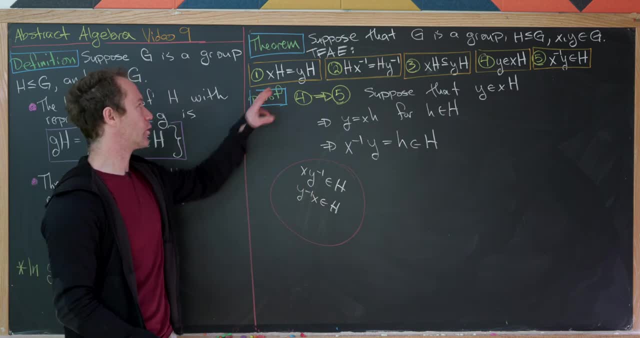 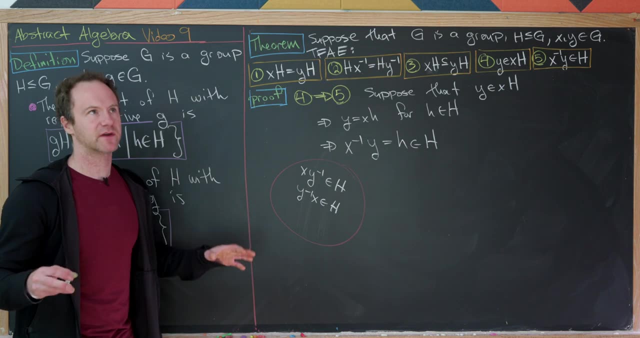 Okay, so let's just keep in mind that these are also equivalent to XH being equal to YH, even though we would have to like prove them in parallel. But the proofs are so similar that we're not going to want them. 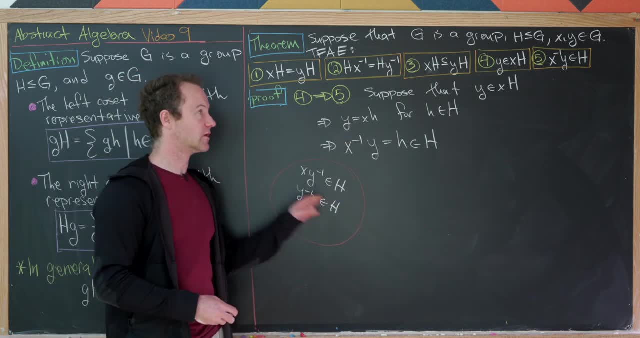 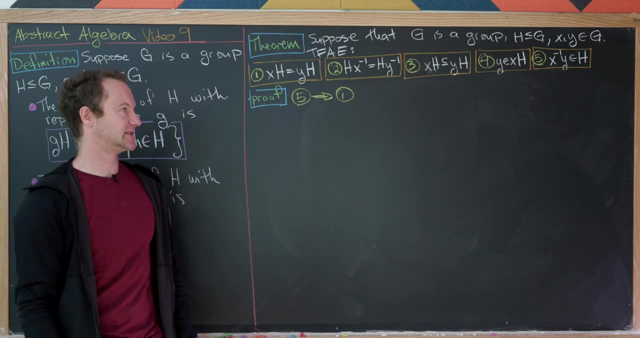 worry about it. Now let's move on to the final part of this loop that 5 implies 1. So to finish our looping argument we will now prove that statement 5 implies statement 1. So let's maybe get started. Let's suppose that X 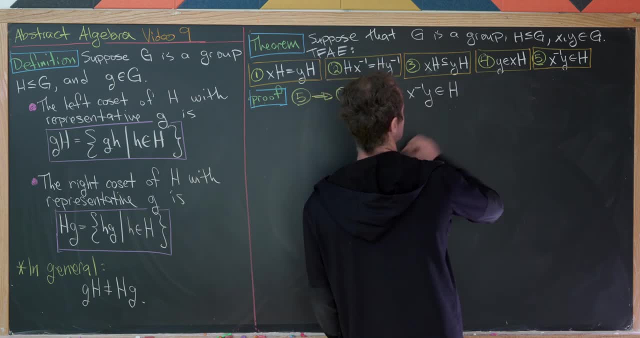 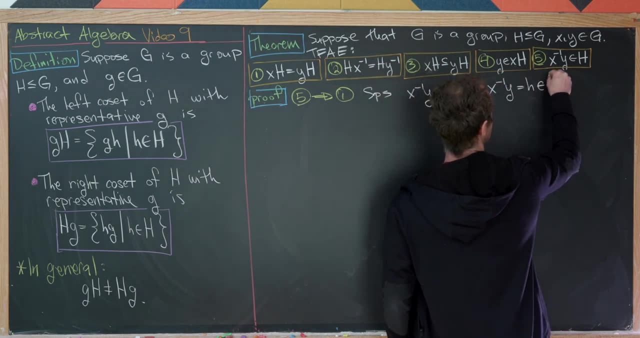 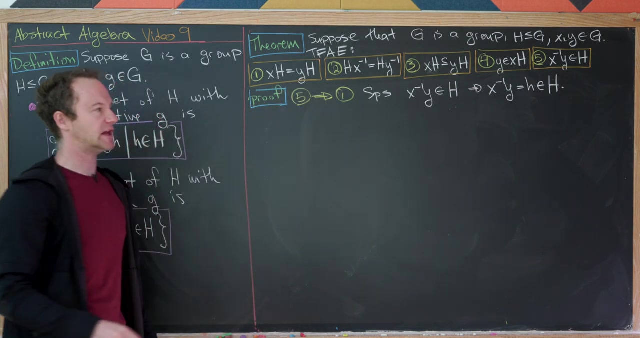 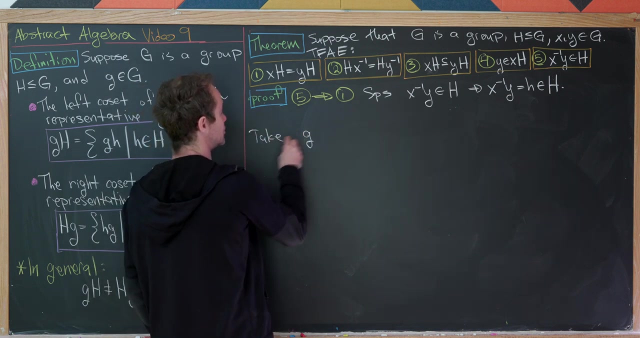 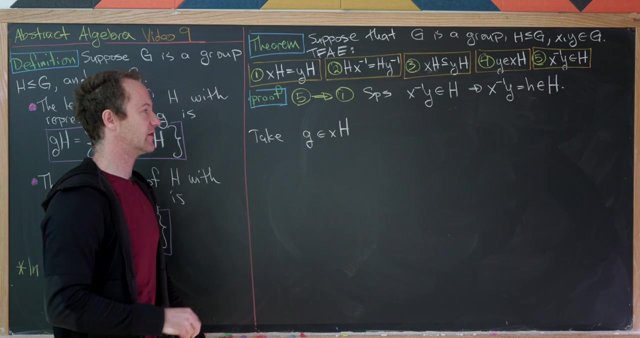 inverse Y is an element of H. But let's notice that that's the same thing as saying that X inverse Y equals little h inside of big H. OK but then now we want to prove that these two cosets are equal, and we'll do that by doubleset containment again. Let's also maybe take an element G from Xh and we'd like to end with G being inside of Yh. And we'll use this fact along the way. Well that's howom let's image that here. Let's imagine that we want two codes 've a bit lower than 1.6 and the second code becomes m or 0. e. and like that we then know this is x. and so for the got do we go our而且 we're going to award 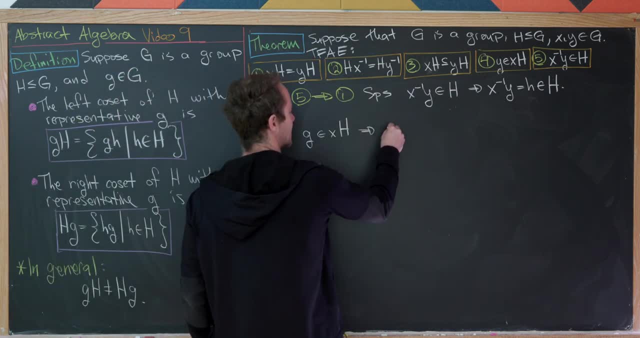 Okay so let's maybe get to it. So this means that little g is equal to x times h naught for h naught 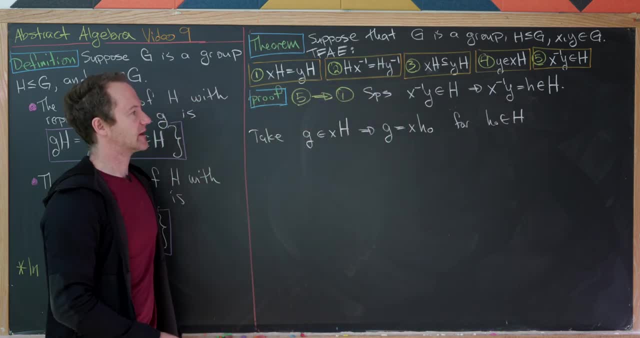 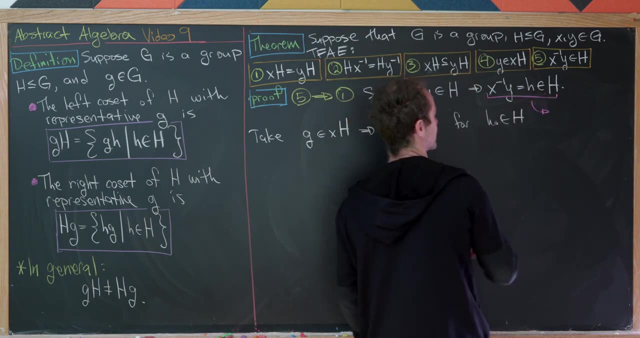 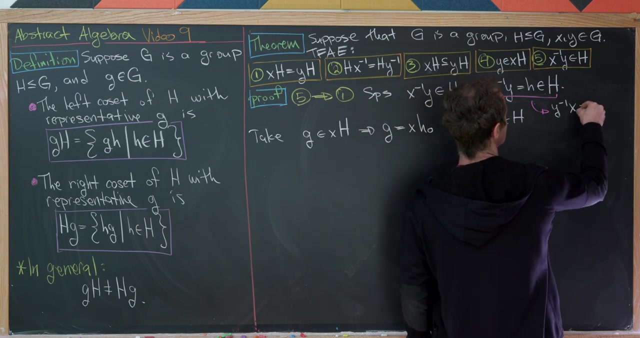 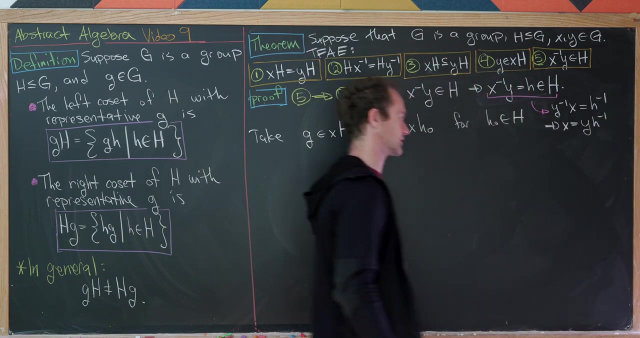 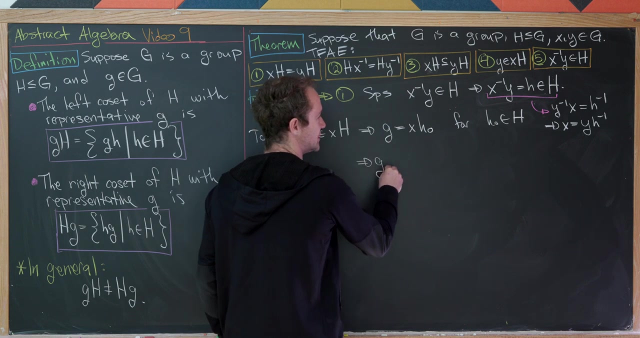 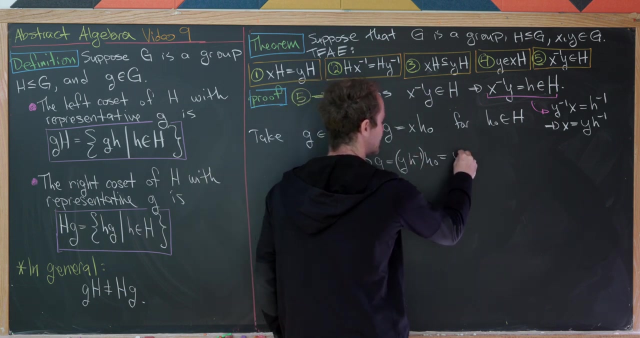 inside of h. So we've got something like that. But now let's go up here to our kind of given statement and invert it to something that's a little bit more helpful here. This is equivalent to saying that y inverse times x is equal to h inverse, but that's the same thing as saying that x is equal to y times h inverse. But now let's replace this x with that y over there, and that's going to give us g is equal to y h inverse times h naught but then we can re-associate to give us h inverse times h naught, and that's going to give us y times h not. 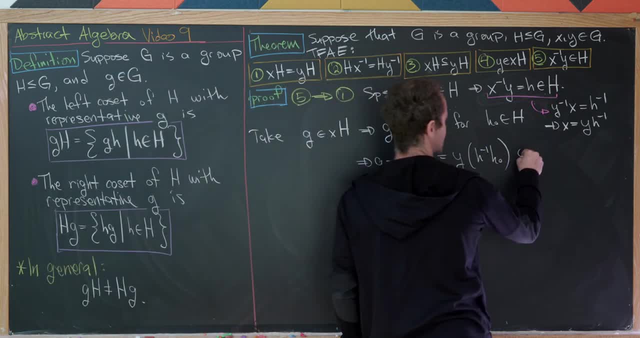 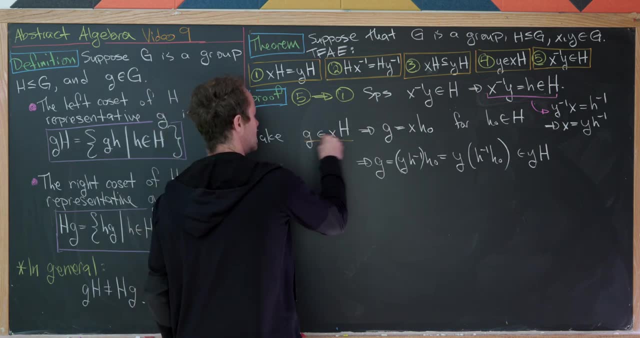 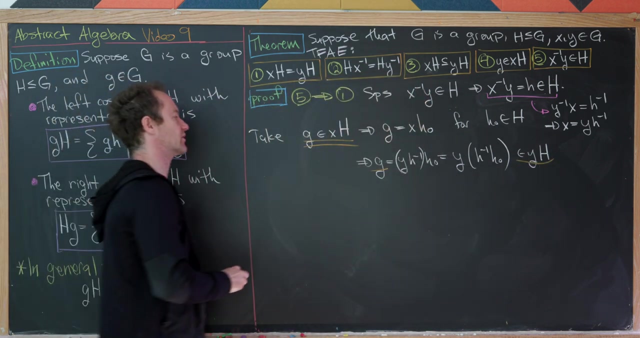 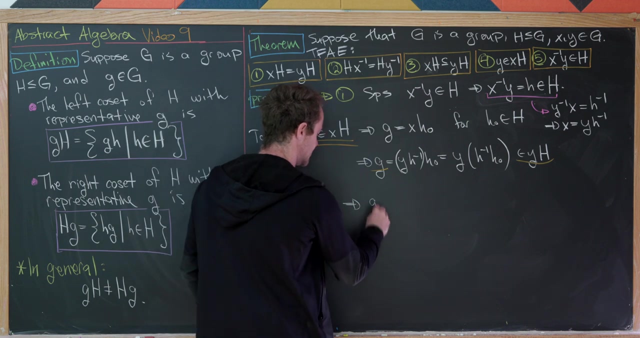 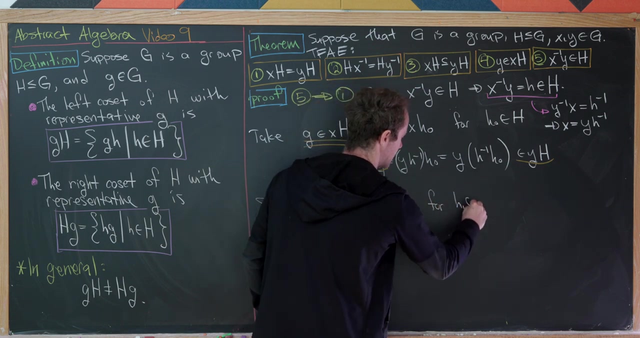 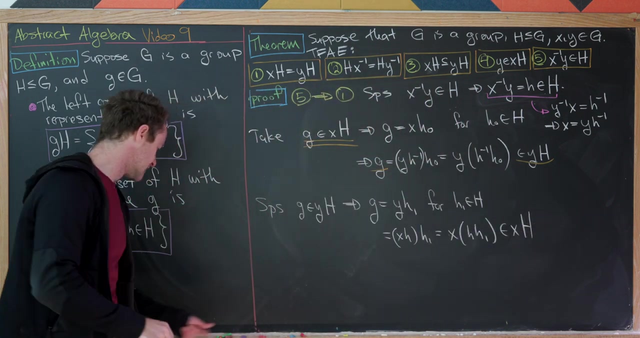 but then we can reassociate to give us h inverse times h not and then we can because H is a subgroup we know this is an element of H so that means this whole thing is an element of YH. So let's see I think we've done one direction. We started here with G is in XH and we ended with G is in YH. Okay so now let's do the other direction. So now let's suppose that G is an element of YH but that means that G is equal to Y times little h, maybe we'll call it 1, for H1 in H. But now we can simply replace Y with X times H given just left multiplying this by X. So let's do that. This is going to be X times H times H1 which is X times H times H1 which is clearly in the coset XH. So let's see here. 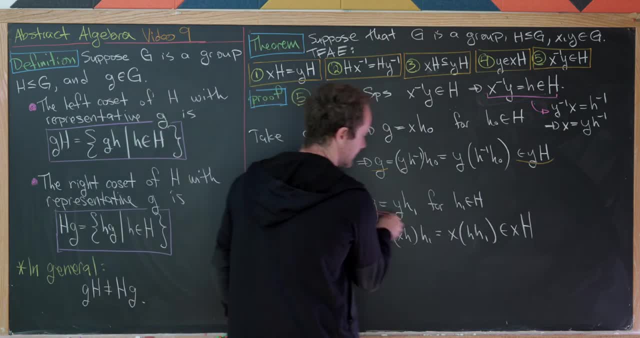 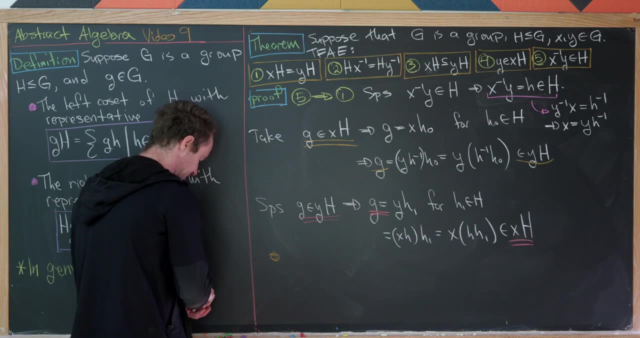 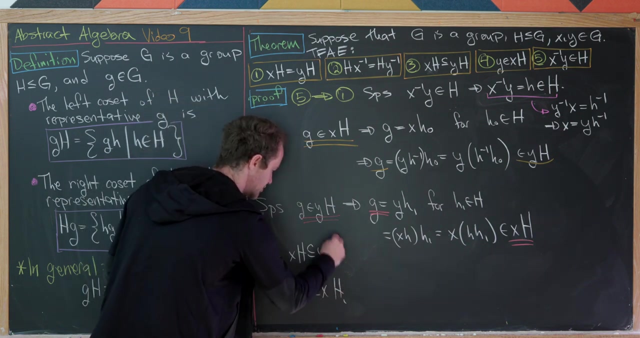 We started with G is in YH and we ended with G is in XH. So this string of orange inclusions gives us one set containment that XH is a subset of YH and then this string of red arguments give us gives us the other inclusion so YH is a subset of XH. So putting these together we see that XH is equal to YH. 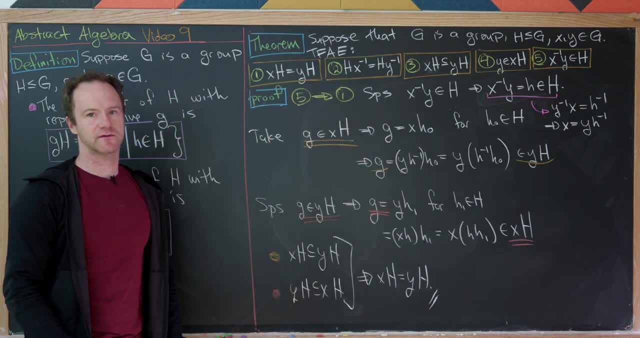 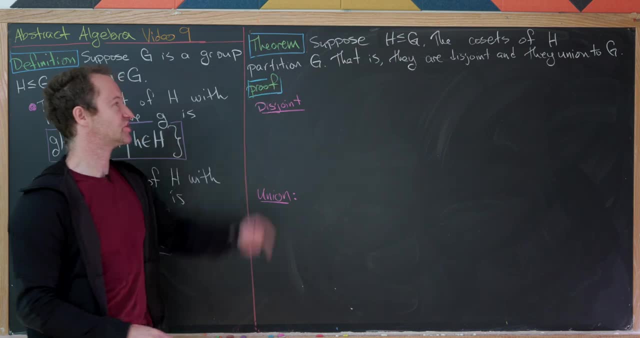 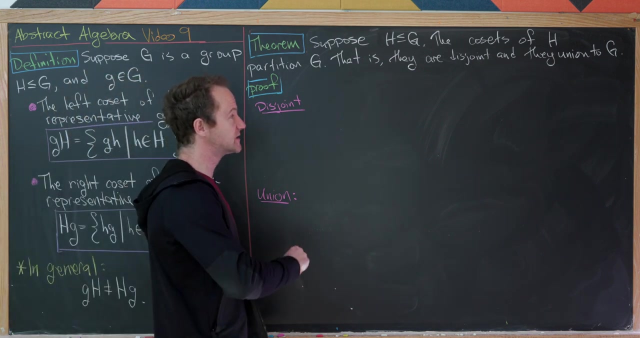 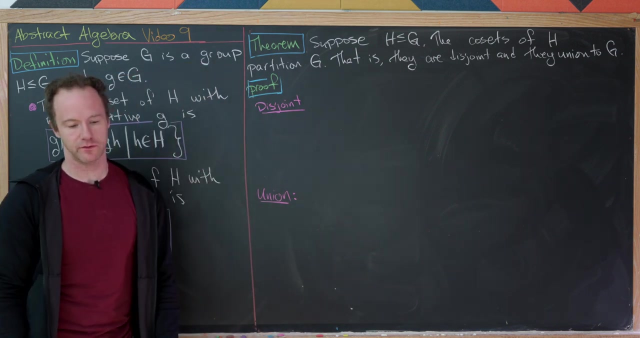 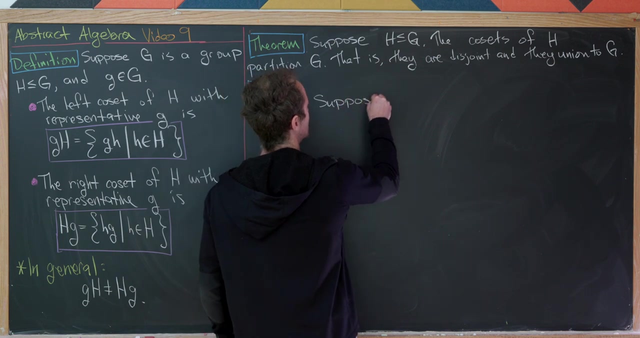 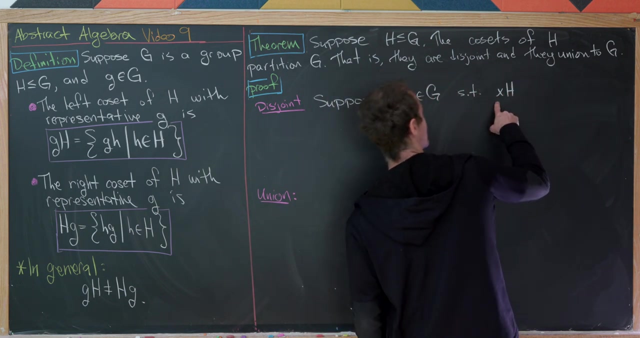 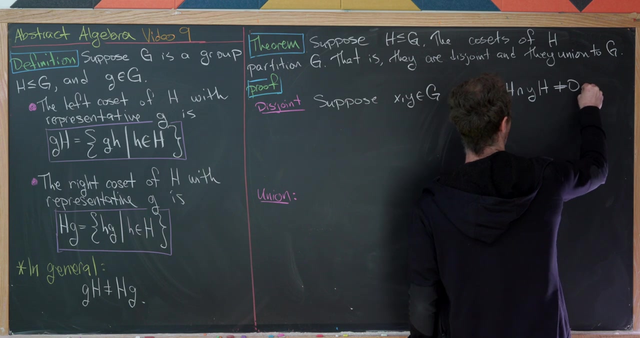 Which is exactly what's needed to finish this proof off. Now we're going to prove a result that we alluded to earlier and that is that the cosets of a subgroup partition a group. Well what do I mean by partition a group? Well that's a fancy way to say that the cosets of a subgroup are disjoint and they union to the whole group. Okay so let's first prove that they are disjoint. So let's suppose we have two elements X and Y inside the group such that the coset with representative X intersect with the coset with representative Y is non-empty. 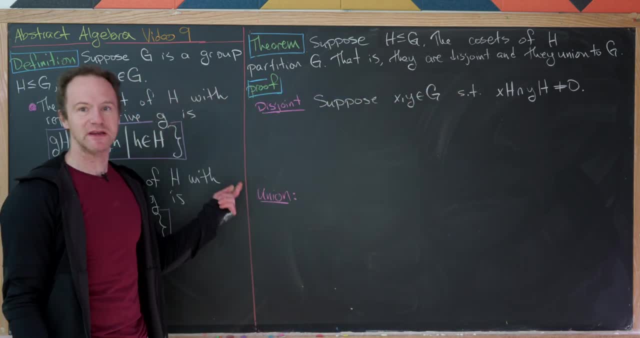 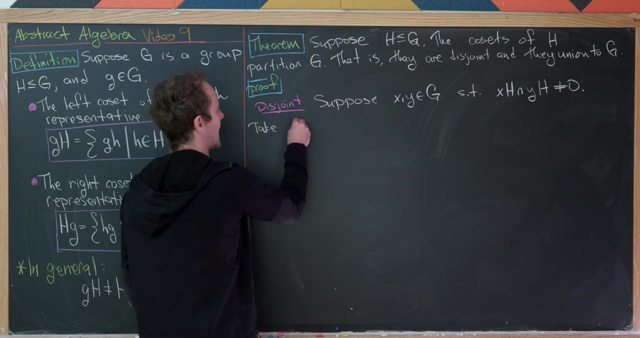 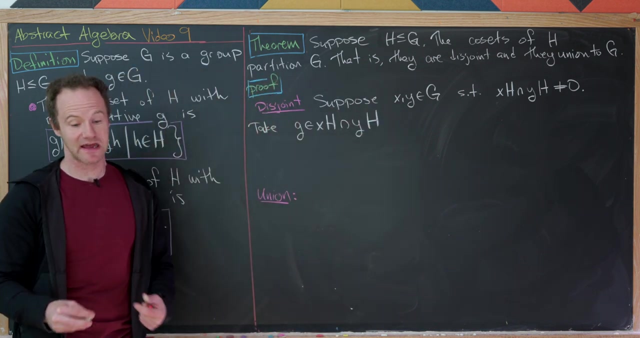 Okay so if it's non-empty then what we should be aiming for is that this means that the two cosets are the same. And that will prove that the cosets are either disjoint or they are the same. I guess like here I'm proving this for left cosets but in complete parallelity you could prove this for right cosets as well but I won't do that here. Okay so like I said let's suppose that happens but if that's non-empty we can take an element little g inside of their intersection. Well that's what it means for them to be non-empty. They contain at least one element. Okay but let's notice that means that they are disjoint and they union to each other. 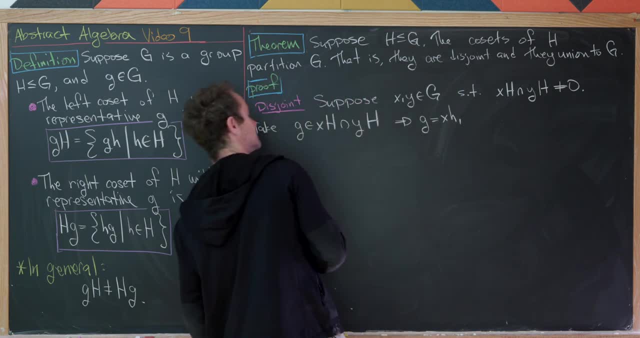 So what we can do is that we can write g as a multiple of X so X times h1 and we 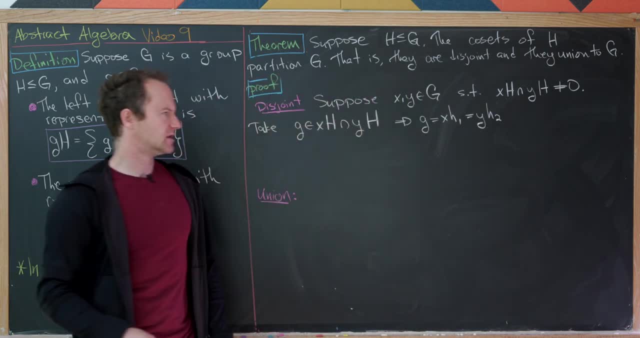 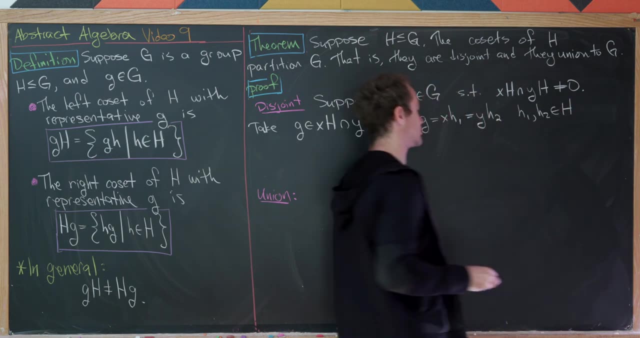 can also write it as a multiple of Y. Let's say Y times h2 and h1 and h2 are elements of H. Okay nice. But now let's focus on this equation that we've just 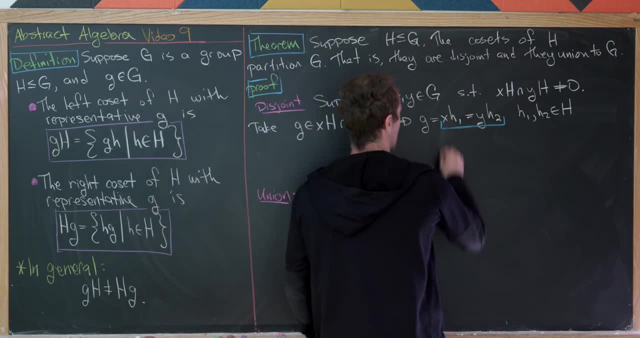 built involving X and Y. And let's maybe try to mold it into something we saw on the previous board. 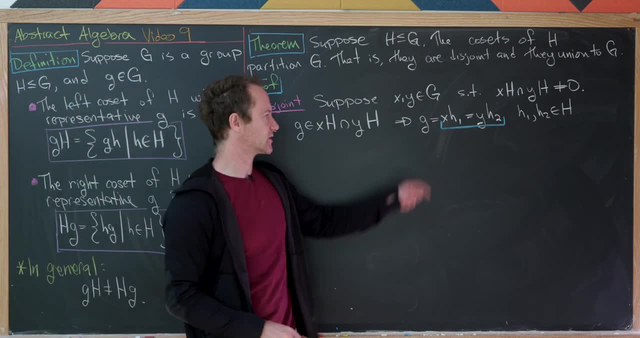 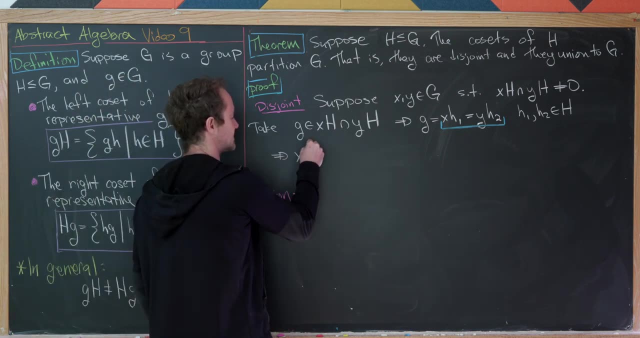 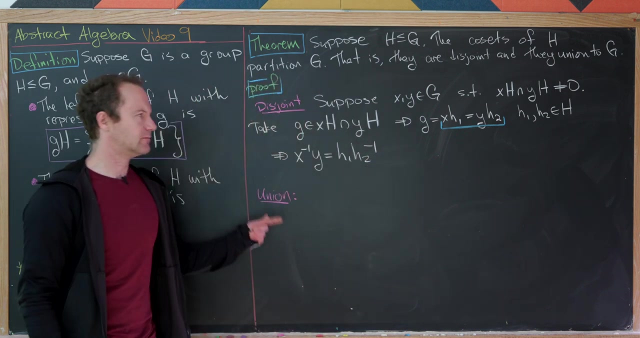 Let's left multiply by X inverse and perhaps we'll right multiply by h2 inverse. So that's going to give us X inverse Y equals h1 h2 inverse. Again by the appropriate left and right multiplications that I described 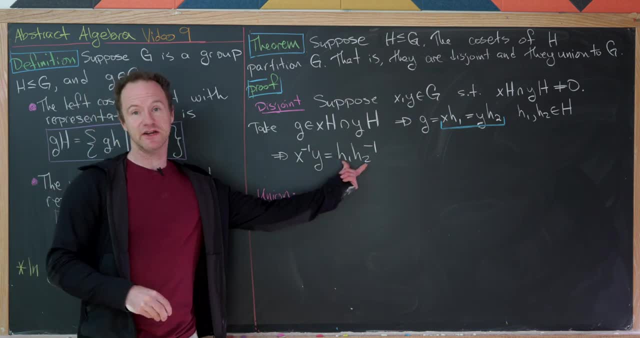 verbally. But this is a combination of things in H so that means it's inside of H as well because H is a subgroup. But now we've got 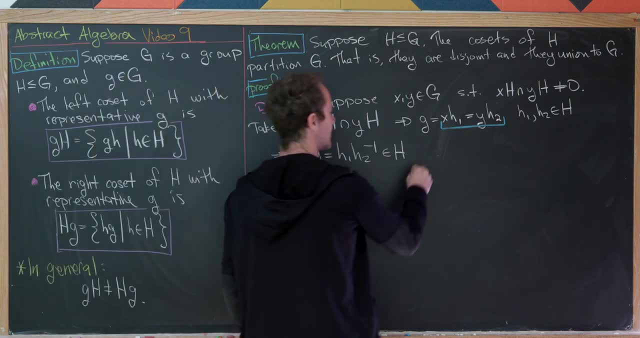 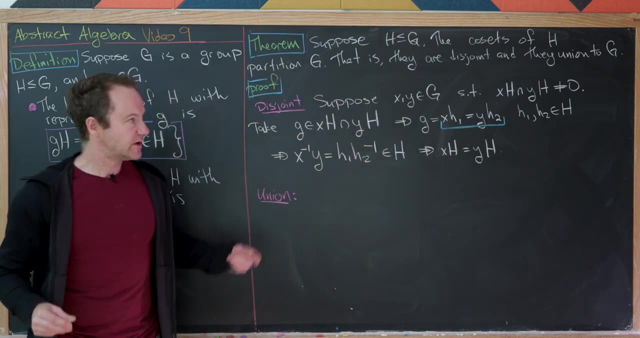 X inverse Y is inside of H. But remember that was one of our equivalent statements to X H equals Y H. And so now we've done it. This means that cosets are 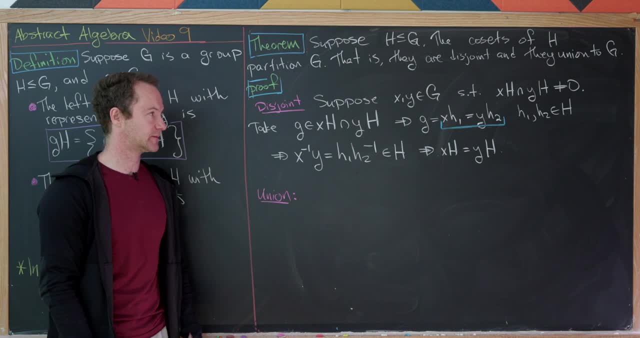 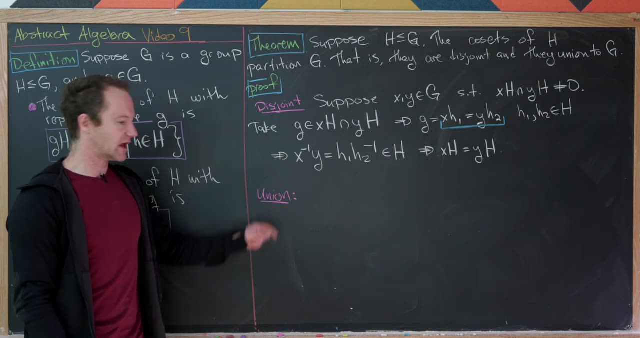 either equal to each other or they are disjoint. So if they contain one element in common then they're the same coset. Okay so now let's show that they union 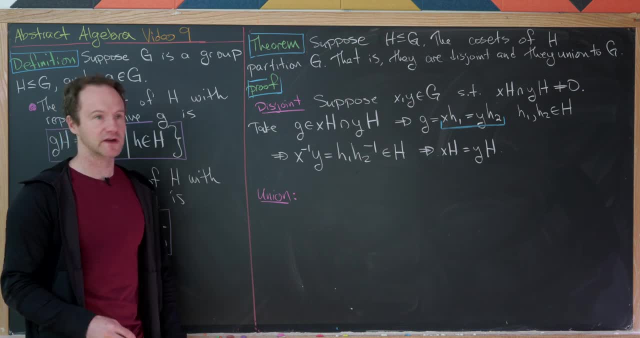 to G. Okay and this is like really quick as well. 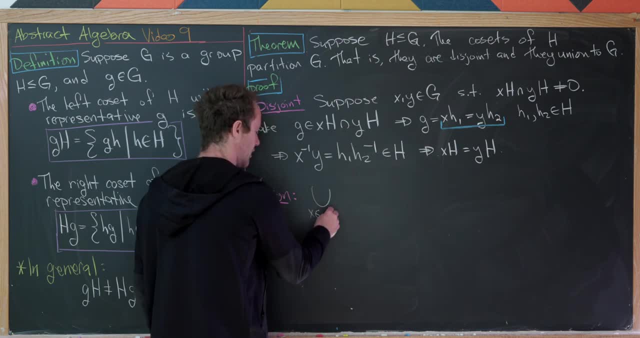 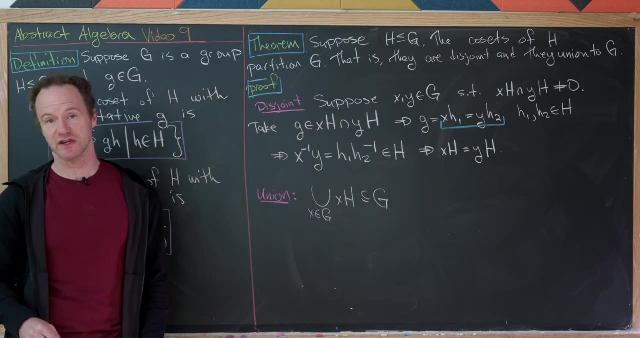 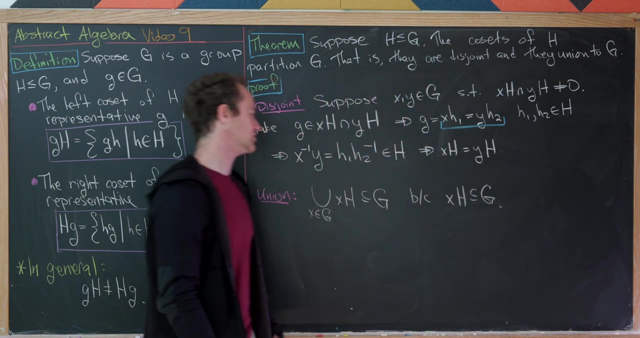 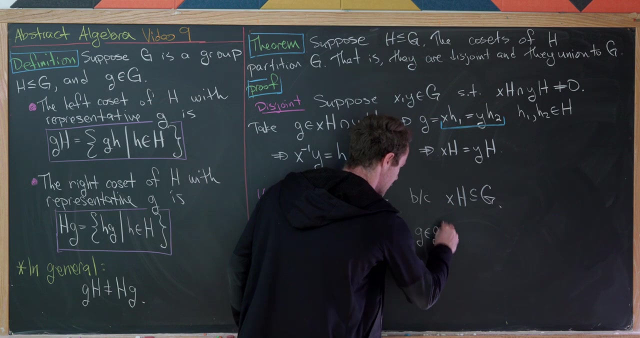 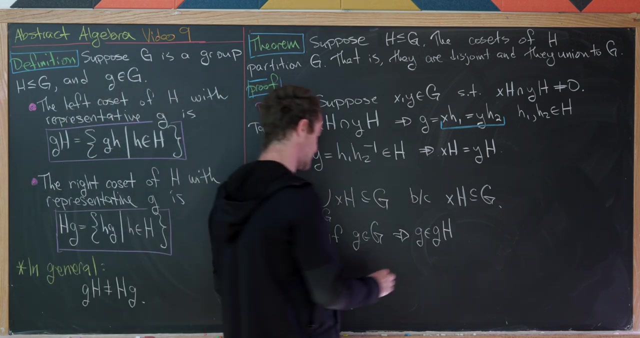 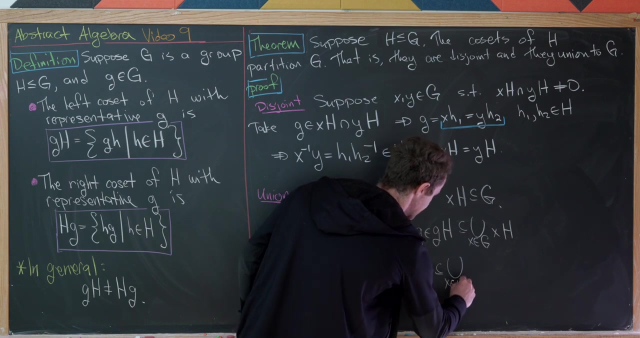 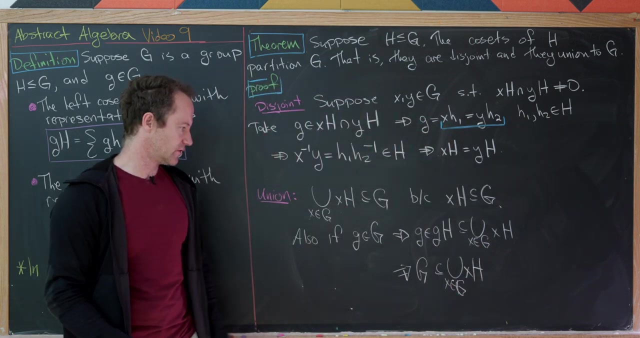 So let's notice if we take the union over all X in G of the cosets X H that's most definitely going to be a subset of G. And why is that well that's because X H itself is a subset of G. So if you union a bunch of subsets of G you will get a subset of G. Now let's also notice that if little g is in G, but now we've got little g is inside of its own coset gh but its own coset is a subset of all of the union of the subsets so this is a subset of the union over all x in g of xh but that tells us that the group g is a subset of this union so let's see let's see what we have put together we have the union of the cosets is a subset of the group and the group is a subset of the union of the cosets 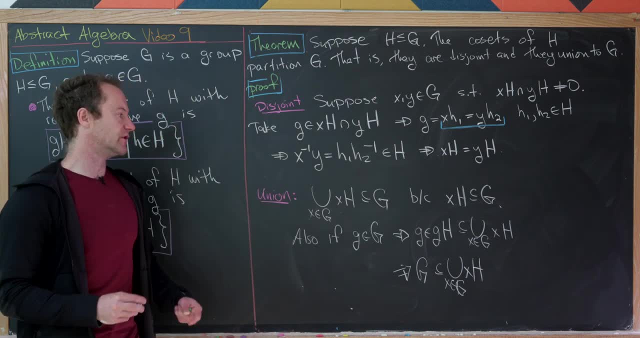 so putting this together by double set inclusion we know that those two have to be equal so now let's move on to another result now we're going to look at the notion of the index of a subgroup 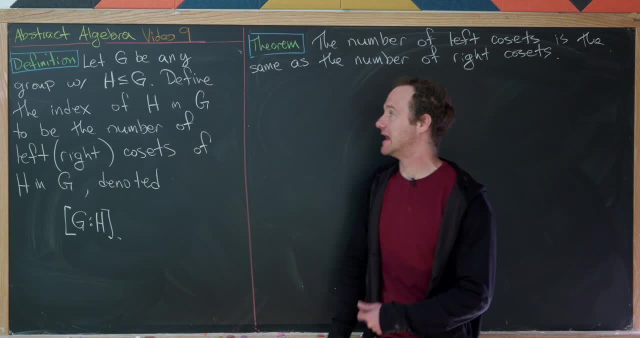 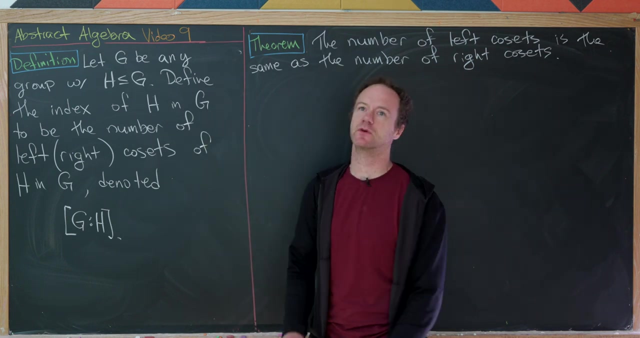 so let's look at our definition so let's let g be any group and h is a subgroup of g we'll define the index of h in g to be the number of left cosets of h in g or the number of right cosets so let's look at the notion of the index of a subgroup so let's look at the notion of the we're about to prove that those are the same numbers so that makes this well defined 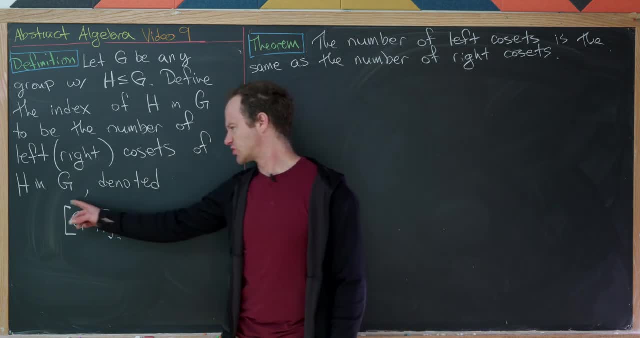 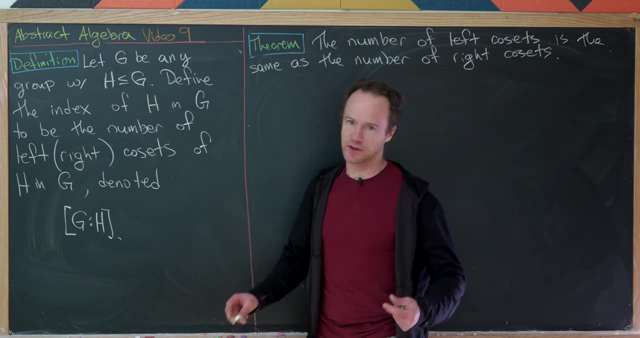 furthermore we have the following notation so i'll just read this as the index of h in g but notice we've got these brackets a g and an h and a colon so that's the quick notation for the index 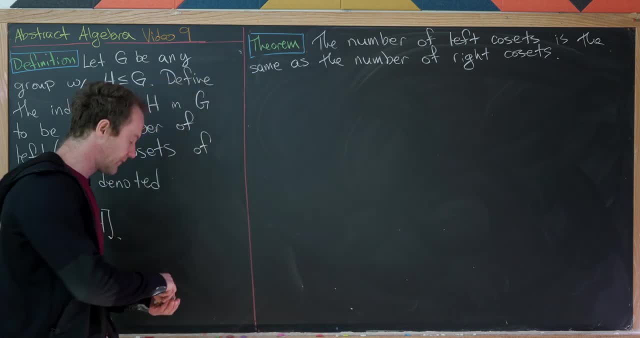 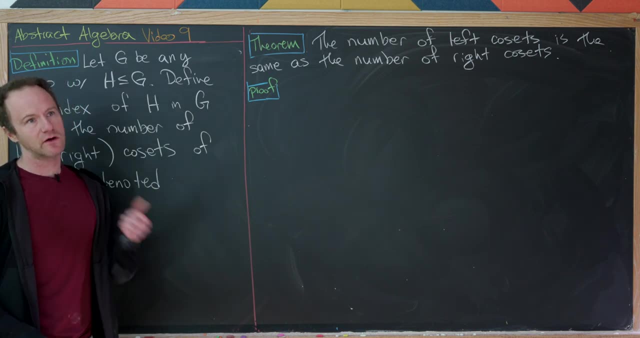 of a subgroup okay so let's see how the proof of this claim goes so how do you prove that the number of elements in two sets are the same well you do it by finding a bijection between 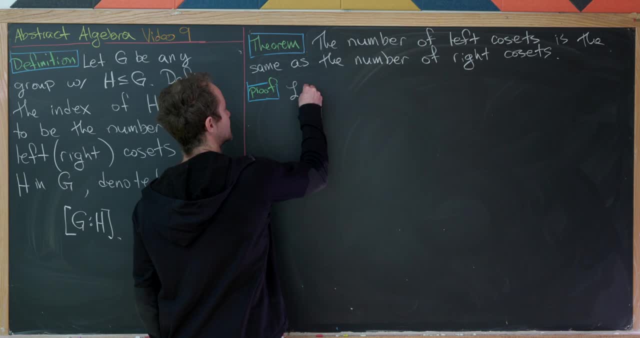 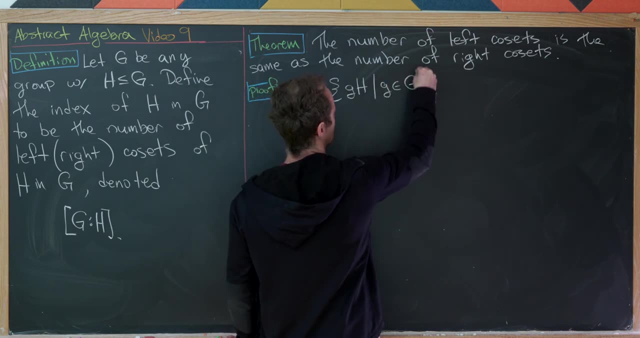 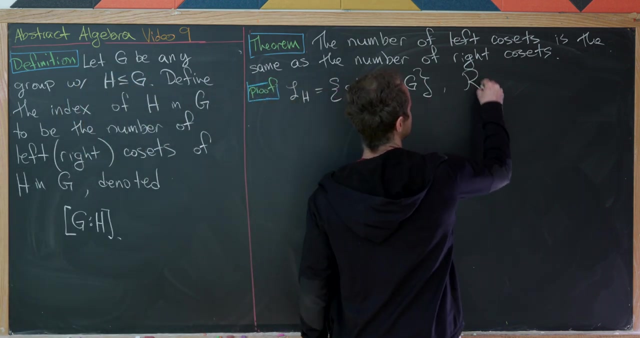 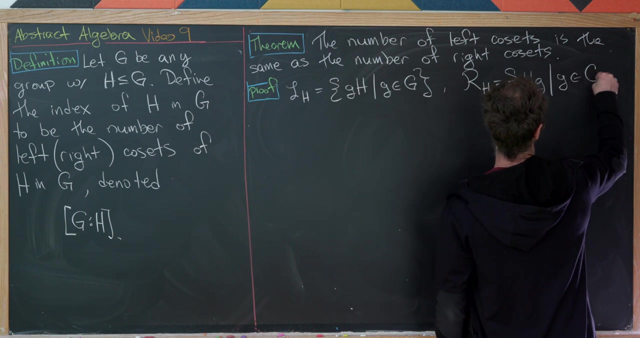 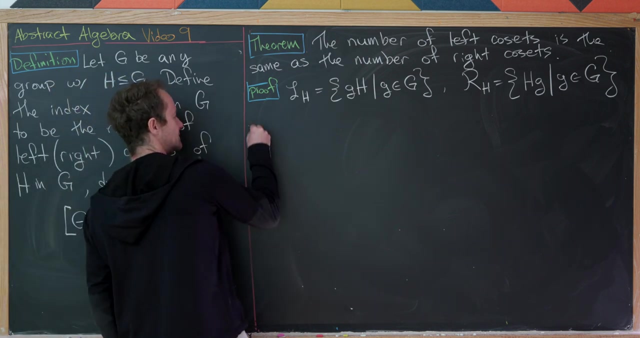 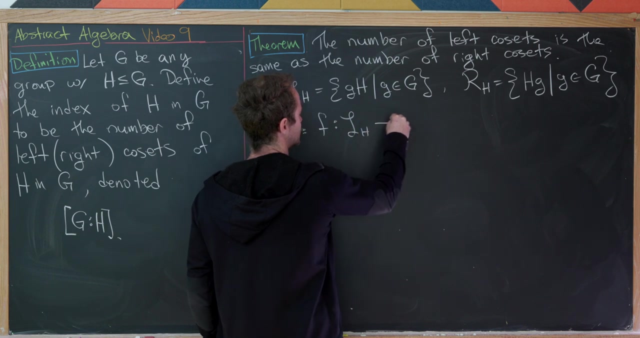 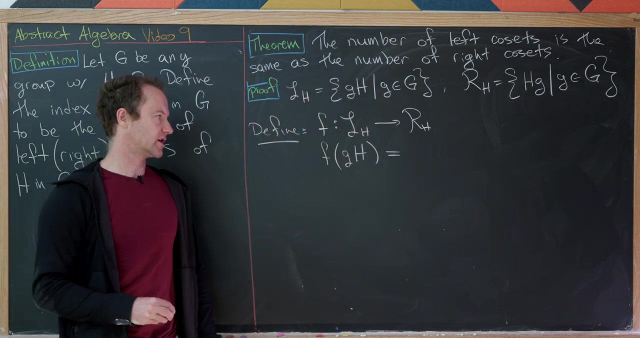 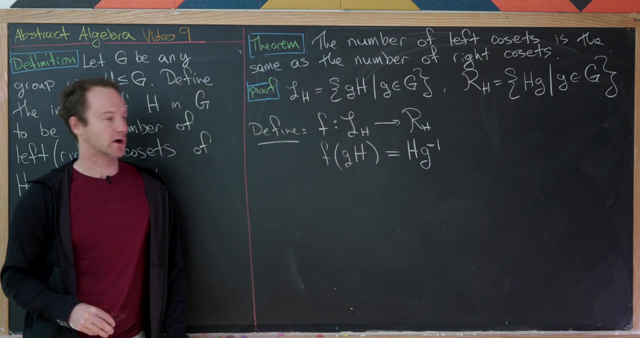 these sets so let's let l sub h be equal to everything of the form little g times h as g runs through all of g so that's the set of all left cosets and then in parallel let's define rh is equal to let's see it'll be everything of the form hg where g runs through all of g so it's all the right cosets now we'd like to find a bijection between these so let's define the following map so we'll call it f and it'll go from lh to rh and what it'll do is it'll take a left coset gh and send it to a right coset but the trick here is you can't send it to the right coset hg you have to send it to the right coset hg inverse otherwise this doesn't work out 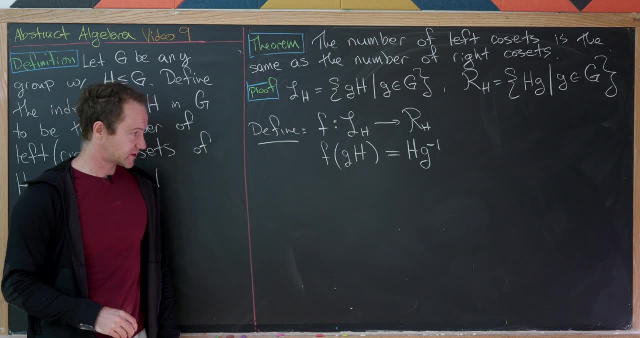 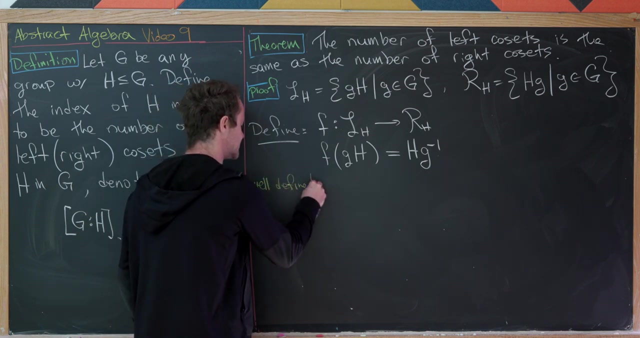 okay so let's maybe notice first that cosets have different representatives and anytime elements of the domain have different representatives you must check that your map is well defined so i think we did this in a previous video we checked that a map was well defined like i said 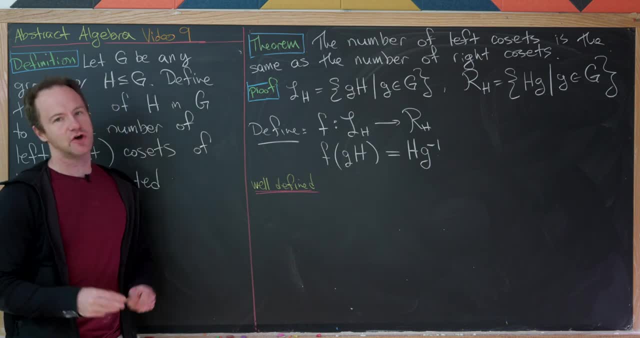 that occurs when the same element of the domain has different names which we saw was possible earlier in this case 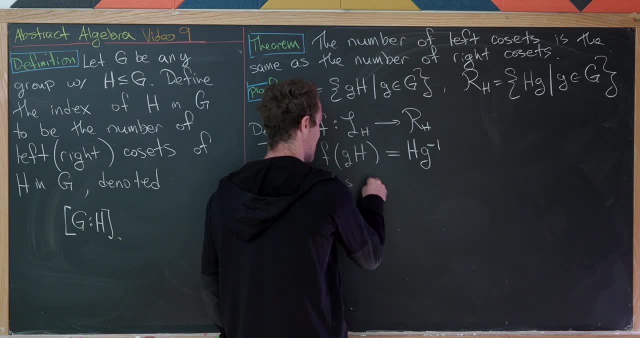 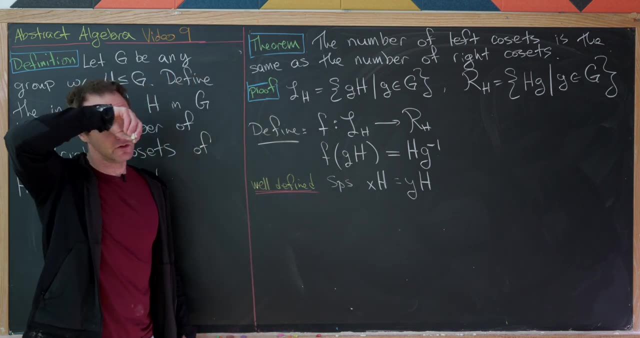 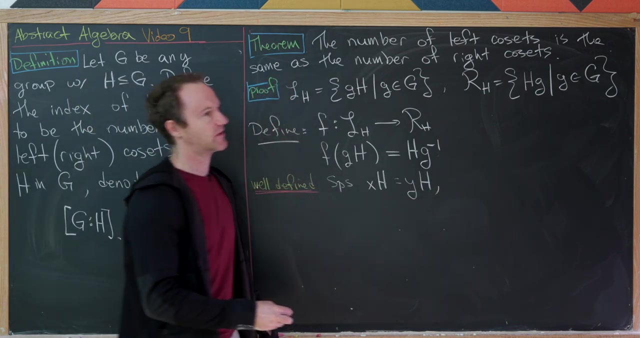 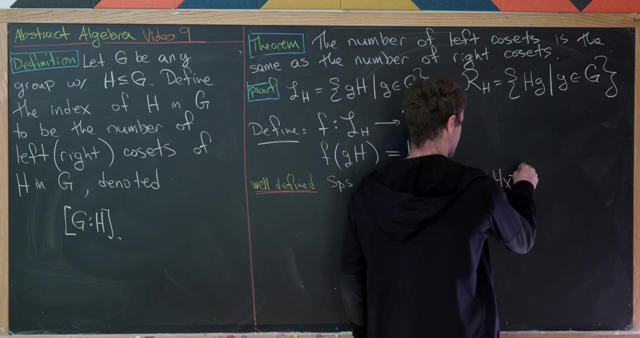 okay so now let's suppose that we have xh is equal to yh with potentially different names and what we'd like to do is show that they have the same output via this function but we prove that big theorem that does all of the heavy lifting here notice that f evaluated at xh is equal to hx inverse but given that xh and yh are the same by that theorem that means that 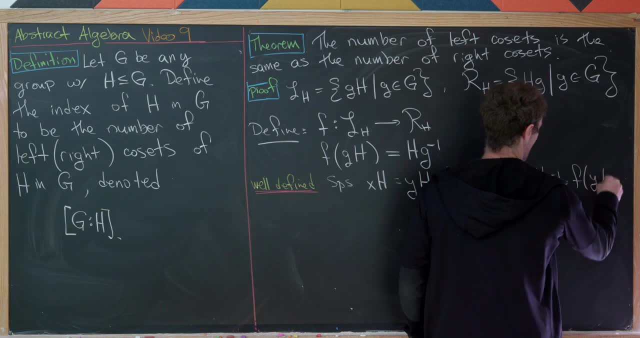 this is equal to hy inverse which is equal to f of yh that's exactly what we need for this thing 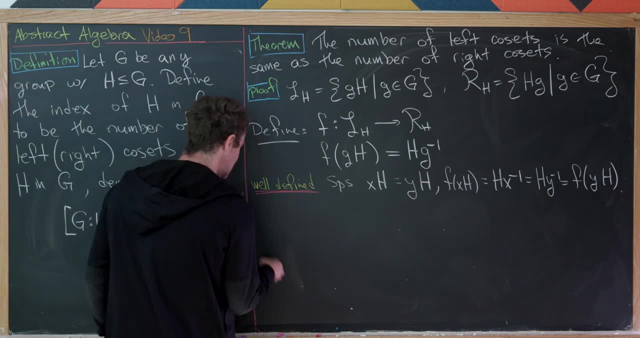 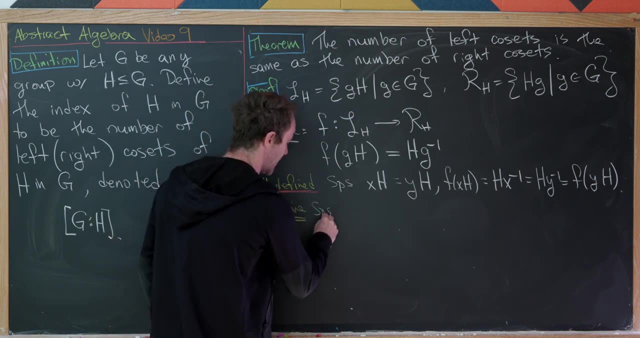 to be well defined so we're good to go there now let's show that it is also injective okay so how could we do that well let's suppose that we have f of xh equals f of yh and we want to show that 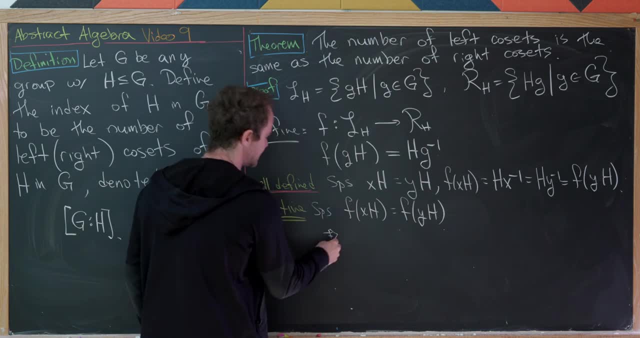 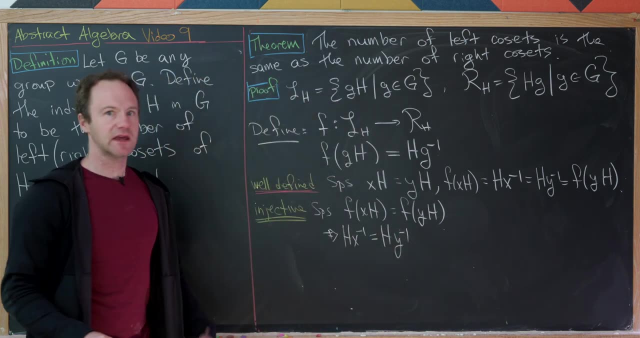 xh and yh are the same coset but notice this it immediately tells us that hx inverse is equal to hy inverse but then again by those equivalent 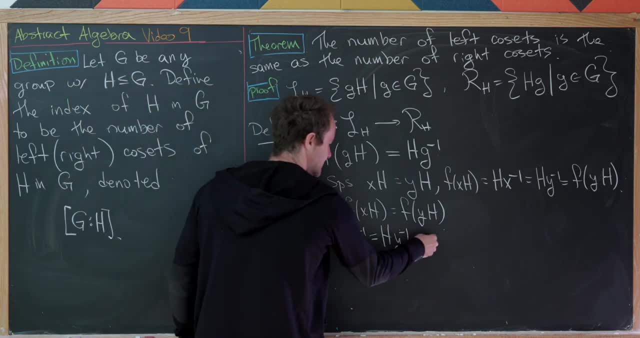 statements of cosets being equal this tells us that xh is equal to yh but that's the injectivity 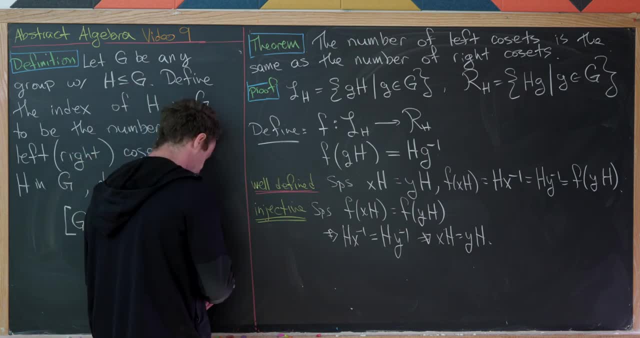 rule there now we need to show that it's surjective as well and that'll finish everything off 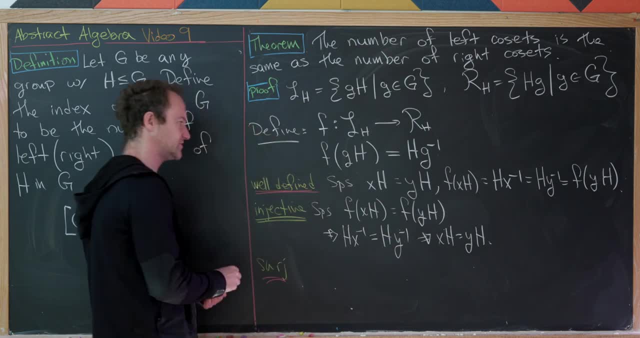 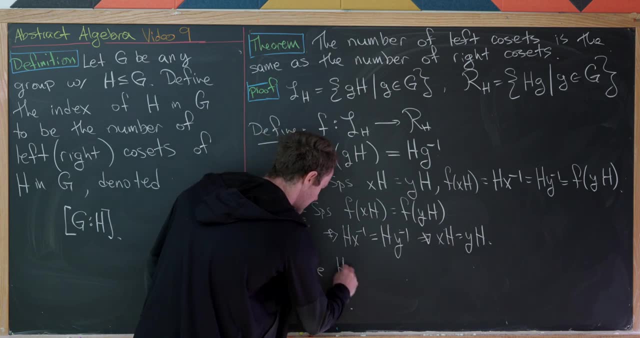 so how might we do that well we just have to find a pre-image for something But let's take an element, which we'll call HG, from the set of right cosets and find something that gets landed on it. 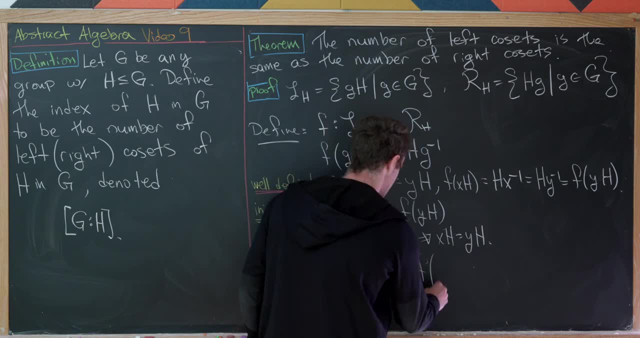 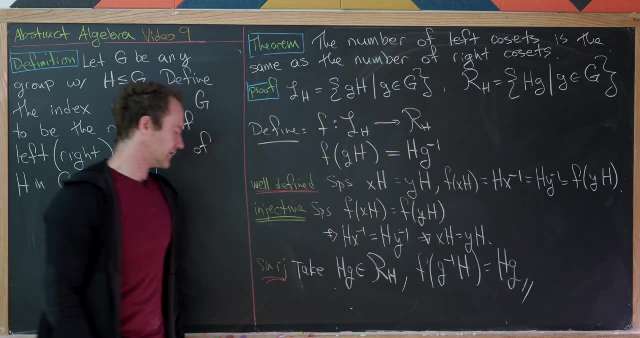 Well, it's not too hard to see that if we take the left coset, G inverse H, it'll land on HG. That's exactly what we need for this thing to be surjective. 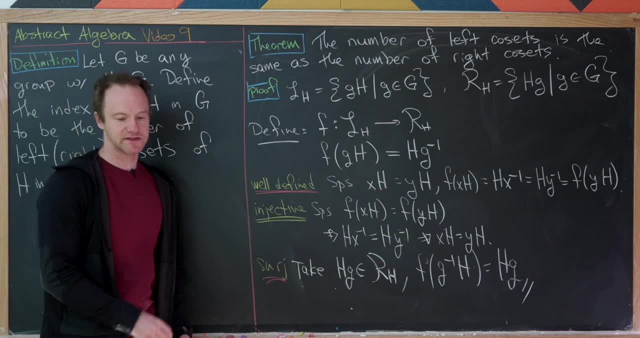 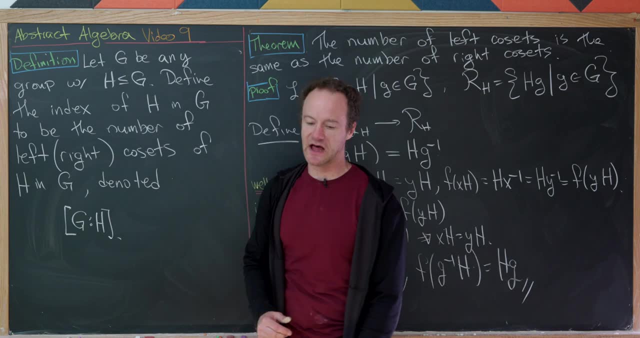 So we've shown that the number of left cosets is the same as the number of right cosets, which shows this idea of the index over here is well-defined. We can count left or right cosets, and we get the same number. 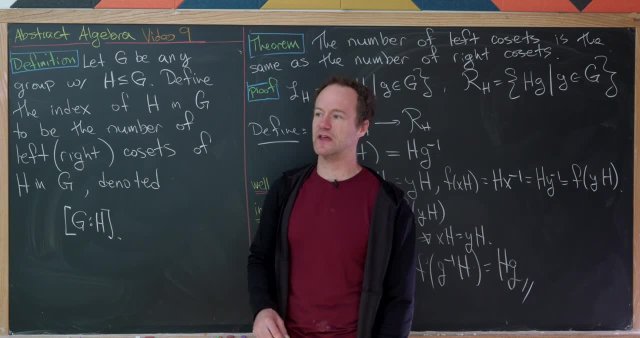 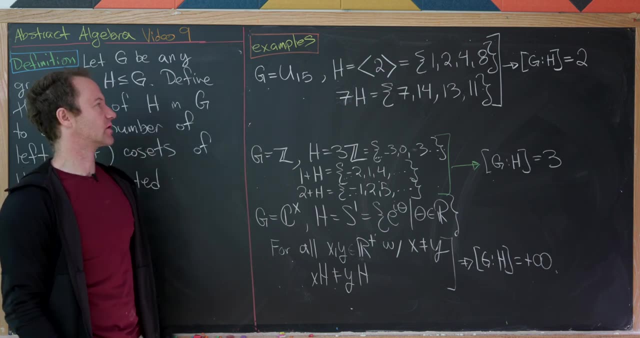 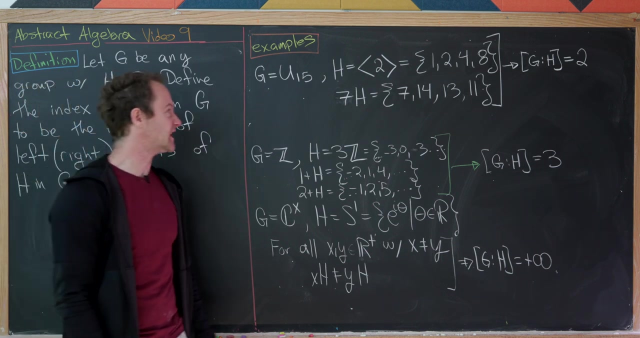 So let's look at a couple of examples of indexes real quick. So here are three examples of finding the index of a subgroup. The first will take our group G to be the group of units mod 15. So let's recall that we'll have eight elements. Because phi of 15 is 8. 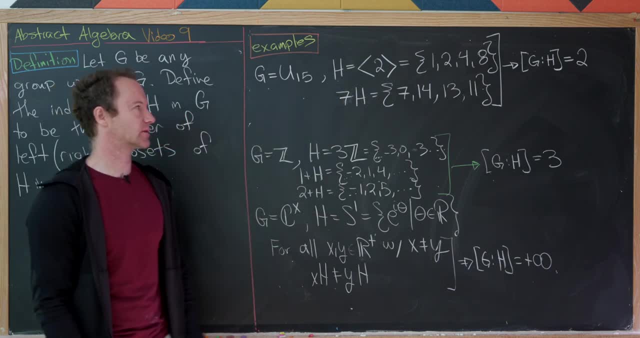 That's Euler's Toscient function. Then we'll take H to be the cyclic subgroup generated by 2. 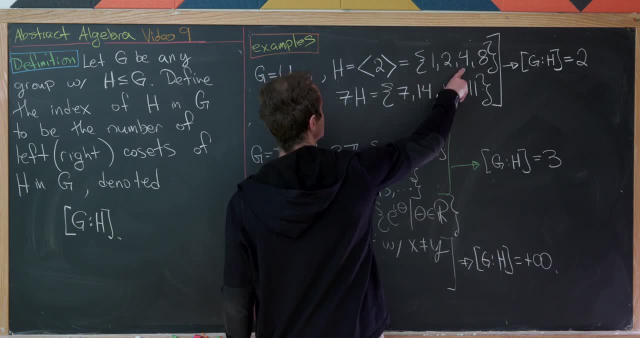 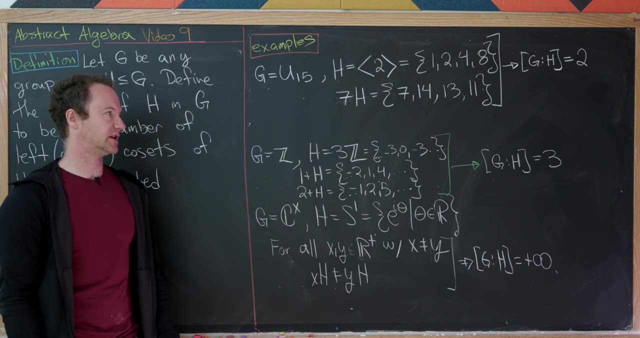 That'll give us 2 to the 0, which is 1, 2 to the 1, 2 to the 2, and 2 to the 3. Notice 2 to the 4 is equal to 16, but that's equal to 1 in U15. 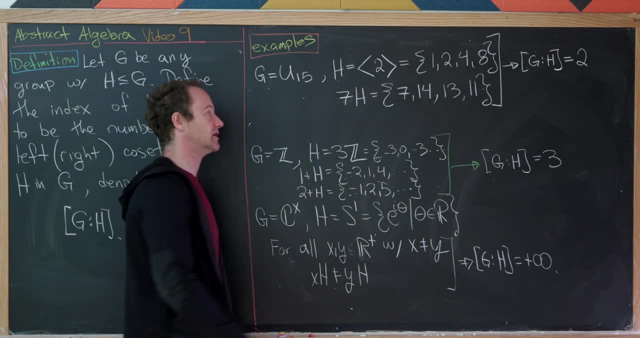 Then let's take an element outside of H, maybe 7, and we'll multiply 7 into each of these. And after reducing mod 15, we get 7. 4. 14. 13. 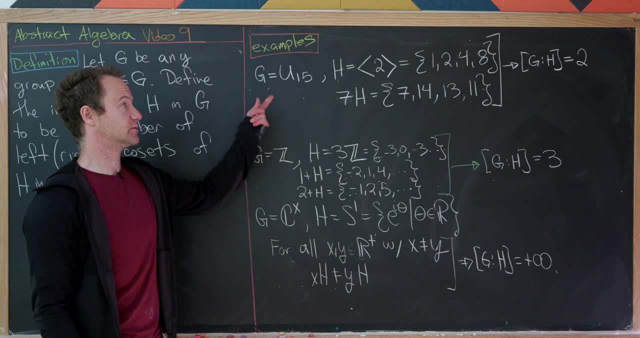 And 11. So those partition the group, which means those are all of the cosets. 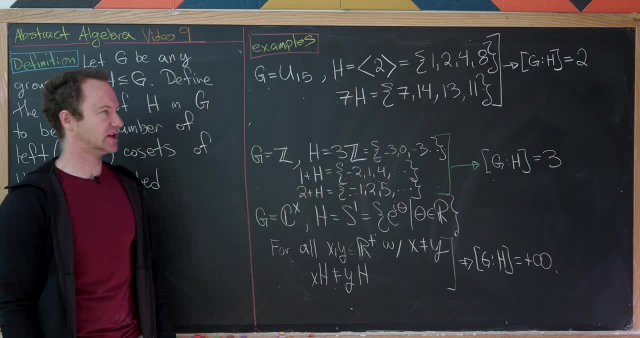 But there are exactly two cosets, so that means the index of G and H in this case is 2. Now let's look at another example. 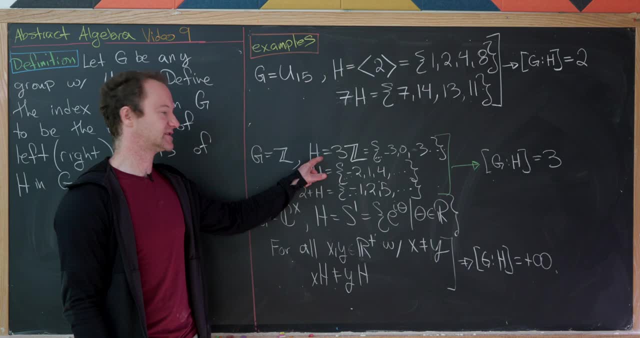 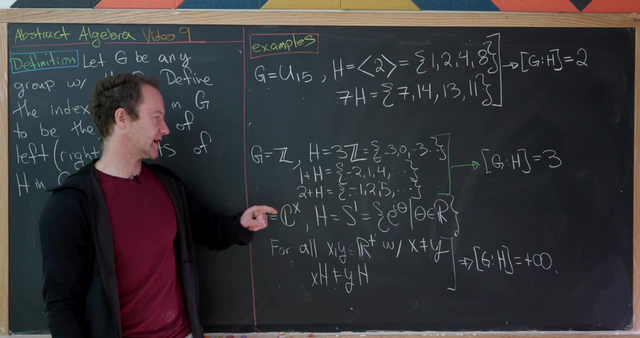 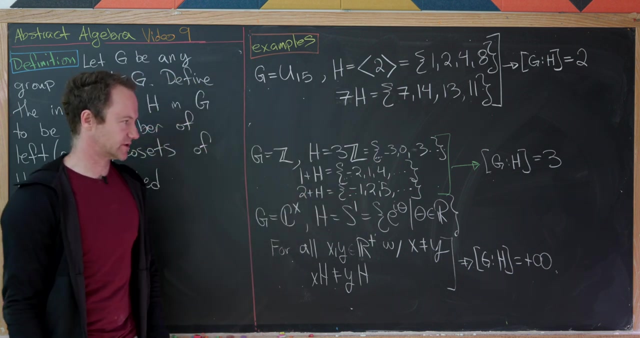 Let's take G to be the integers, and H to be the cyclic group generated by 3 under addition 3Z. So that's all multiples of 3. Let's notice that 1 plus H will contain negative 2, 1, 4, so on and so forth. 2 plus H will be negative 1, 2, 5, so on and so forth. But that's all of the cosets, because all of the integers are contained in one of those sets. 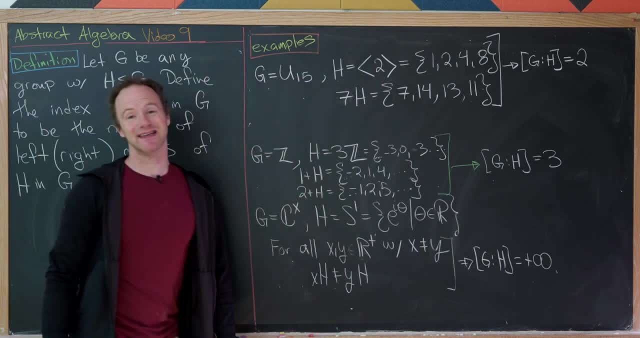 That means the index of G and H in this case is 3. 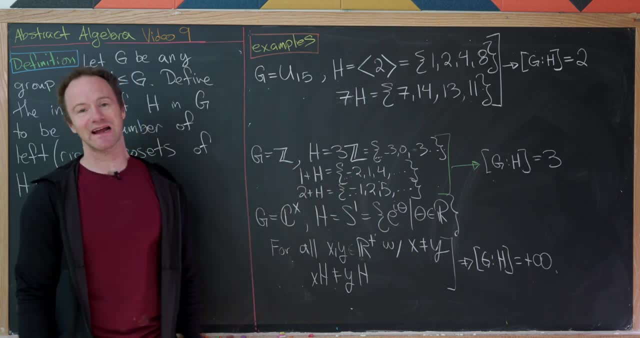 So notice we've got an infinite group with a finite index. So I think that's interesting in itself. 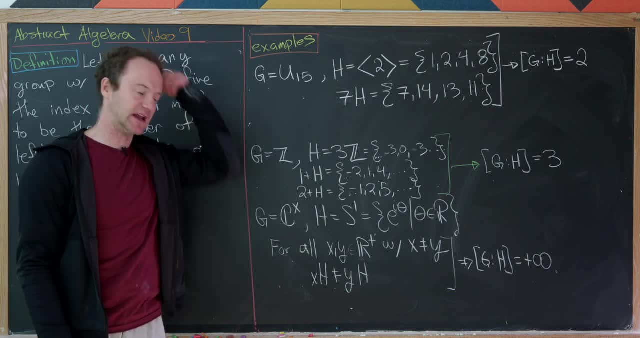 But notice we could also have an infinite group with an infinite index, and that's exhibited by this example. Let's take G to be the infinite group with a finite index. 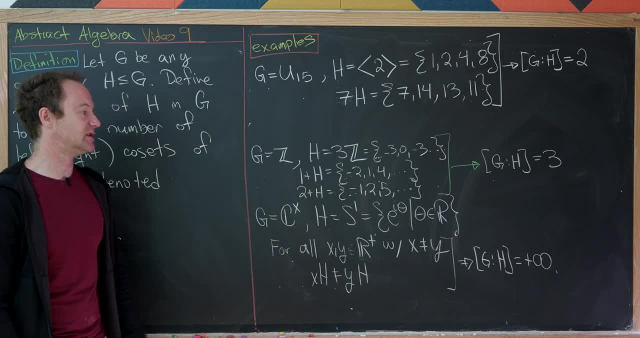 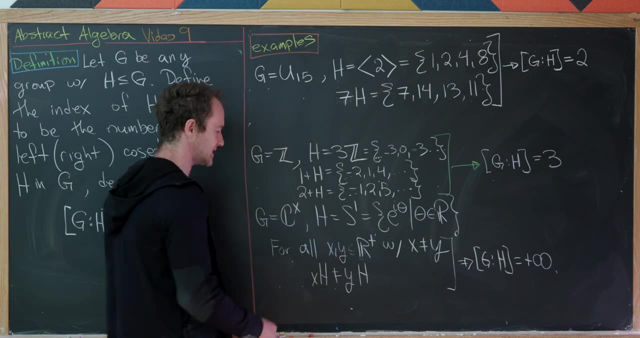 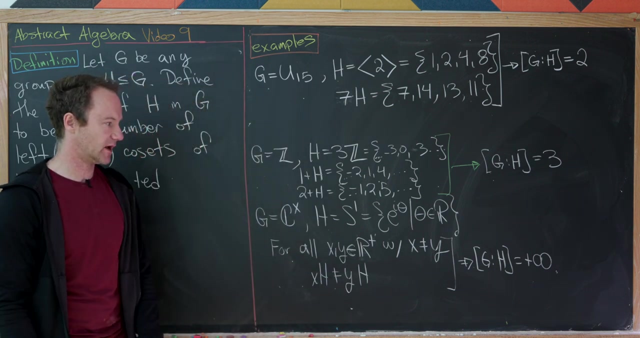 Let's take G to be multiplicative complex numbers, H to be the circle group, as we saw before. And notice for all positive real numbers X and Y, the coset containing X is not equal to the coset containing Y. 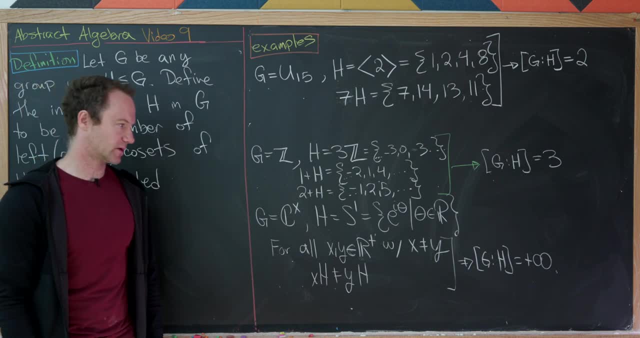 But there are clearly infinitely many positive real numbers, so that means we have infinitely many cosets, which means the index of H and G in this case is infinite. 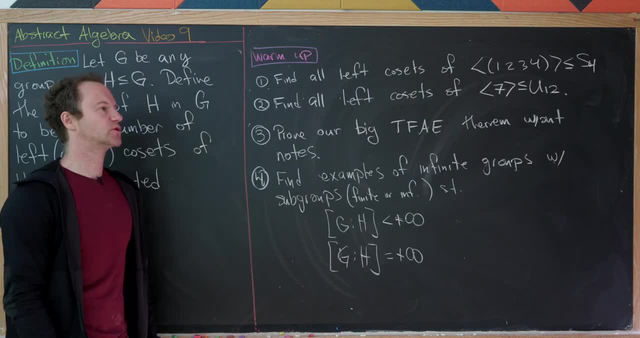 Now I'm going to leave you with some warm-up. Here are three nice warm-up exercises based on what we saw today.